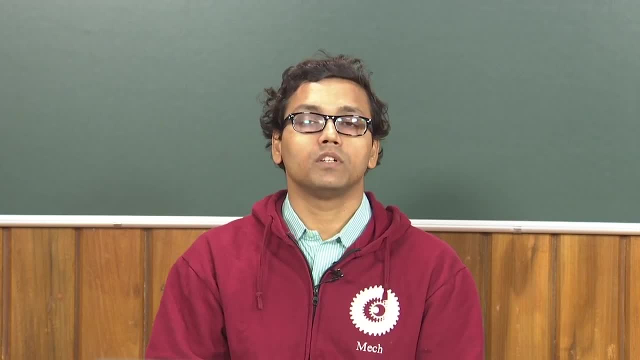 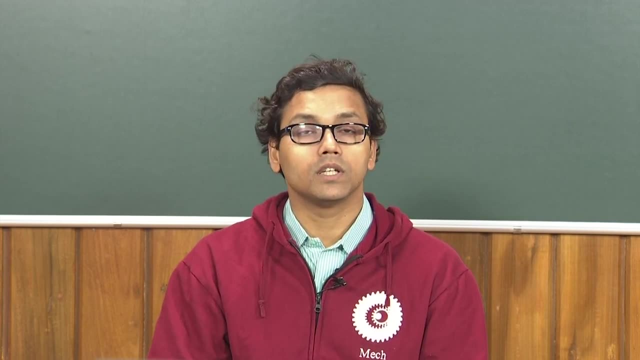 with the analysis of fluid flow. Therefore the term thermal hydraulics is generally used for simultaneous analysis of heat transfer and fluid flow problems and hence in this particular module we are going to look at the heat transfer aspect and also the flow aspects, whenever necessary, of a nuclear 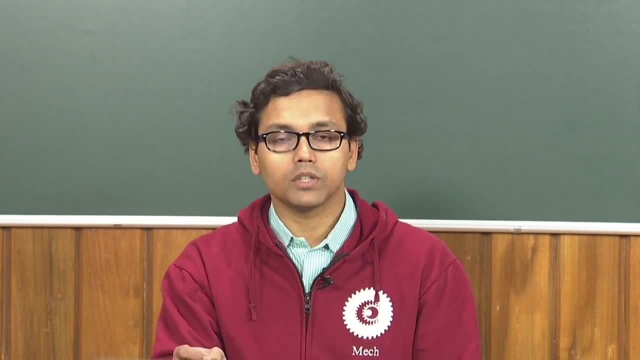 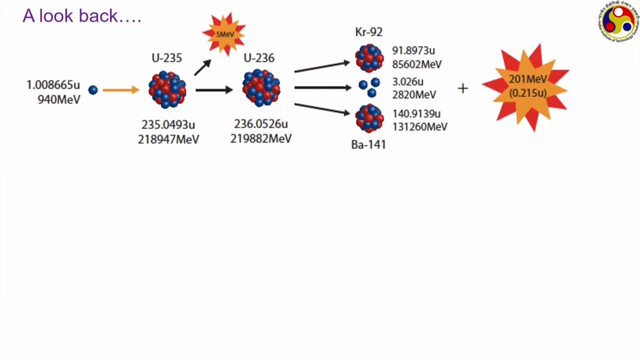 reactor. To start with, just a quick look back at the four modules that we had. like I am taking you back to the first module itself, where this picture was shown. Whenever a neutron or strikes a uranium 235 nucleus, it initially forms a temporary nucleus in the form of uranium 236, and then we have the fission reaction when this intermediate 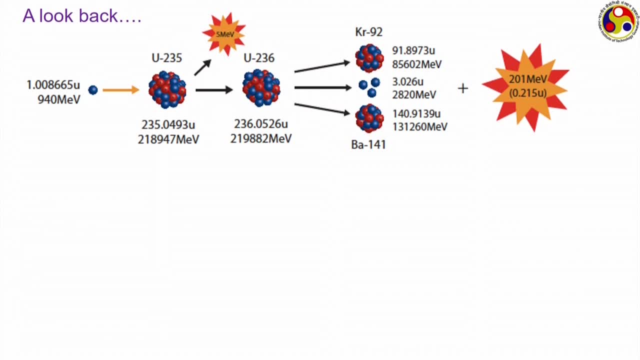 nucleus, or isotope, breaks into two much lighter isotopes. In this case it is krypton 92 and barium 141, plus 3 neutrons, and it is also associated with a large amount of energy In the first module itself. we have learned: whenever such a reactor is formed, it is a 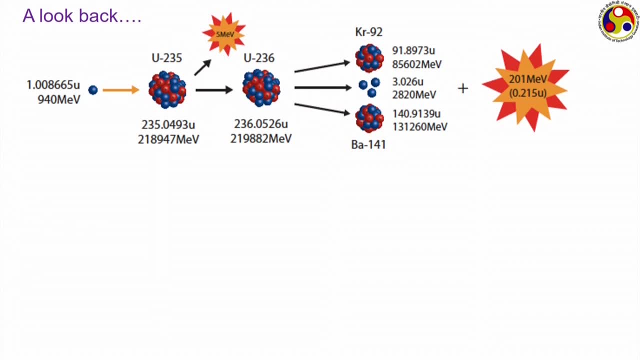 reaction is given without trying to understand the inherent physics of that. We have learned that how to calculate this amount of energy release. We know that whenever we know the values of this mass, we can calculate the mass defect, that is, the mass of combined mass. 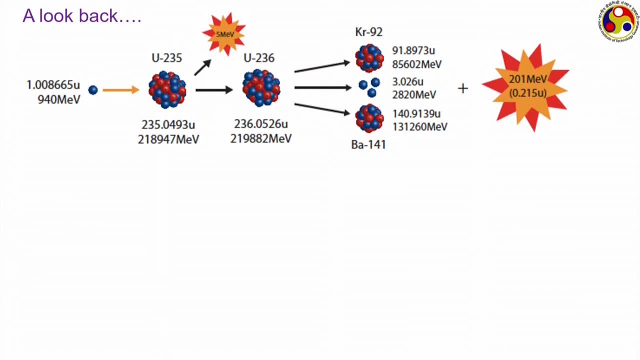 of the products will be generally slightly higher than the combined mass of all these reactants and this difference was termed as the mass defect. and we know the mass defect multiplied by c square, can be related to the total amount of energy that has been released during this reaction. Whenever we are having any reaction, even in 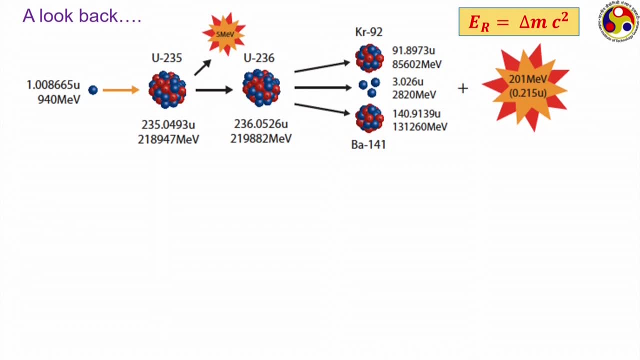 common chemical reactions there is generally small amount of mass defect. but the amount of mass defect that generally we get in a chemical reaction is negligibly small compared to what we get in case of a chemical reaction, And therefore chemical reactions are. then we get in a nuclear reaction, I should say, and that is why in nuclear reaction we get 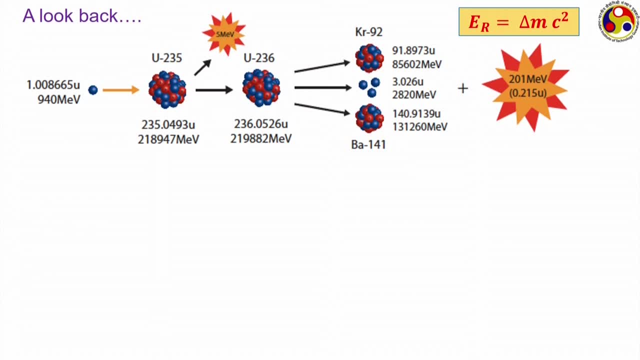 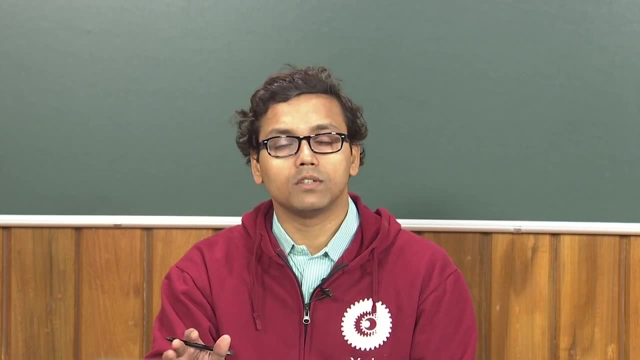 huge amount of energy release, which can be of the order of 10 to the power 6 to 10 to the power 7 times greater compared to a equivalent chemical reaction. So in the first module itself, we have learned how to calculate this amount of energy once. 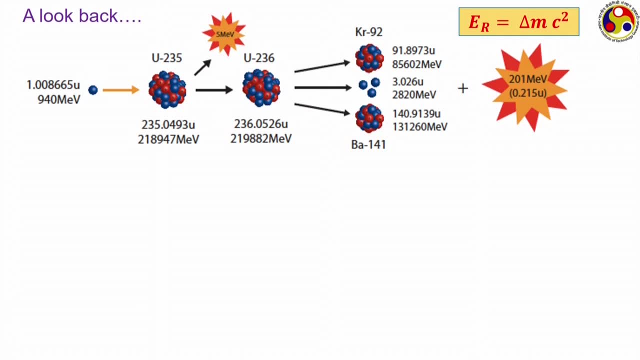 we know the mass of all these components involved. But in the second module we learned that while there are several nucleus which can undergo spontaneous radioactive decay, this particular kind of fission reaction is generally not common, or it does not happen naturally. So rather we have to induce this kind of reaction by striking the nucleus with a suitably charged 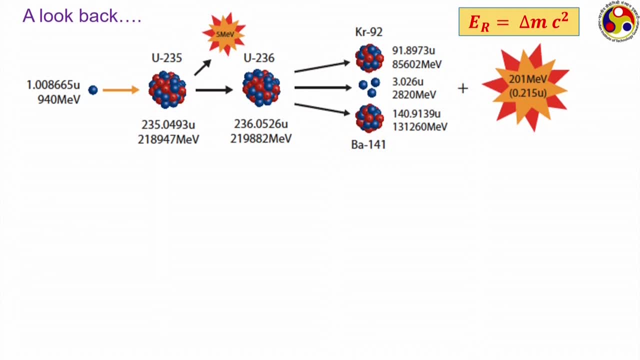 particle which comes under the category of artificial radioactivity, And even when we strike a nucleus with a particle, commonly neutron is the most suitable particle. we can have different kinds of reactions, like we can have scattering, which is associated with both elastic and inelastic collisions. That is, neutron and nucleus with a suitable. 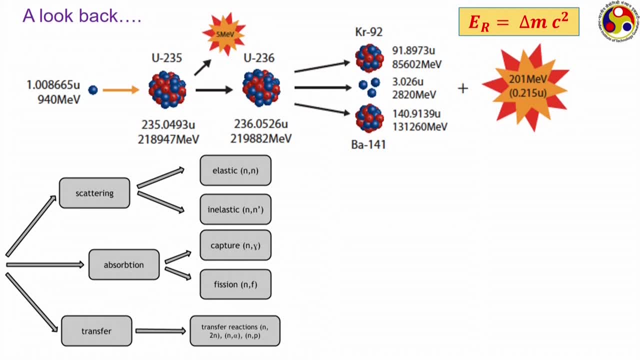 reaction may extend their momentum and energy and can have a perfect conservation of both kinetic energy and momentum in case of an elastic collision. in case of inelastic collision, we have some amount of energy release as well. We can also have some kind of transfer reactions. 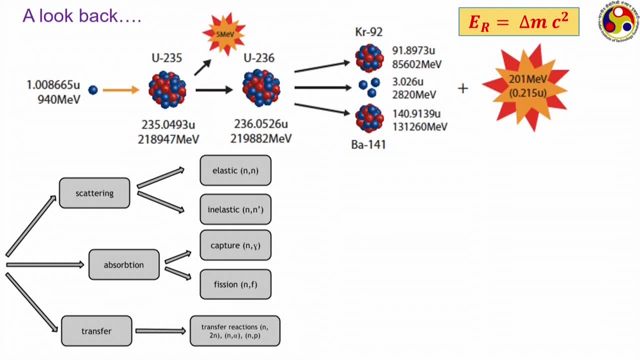 only in very small fraction of total situations we can have the neutron being absorbed in the nucleus. And whenever the neutron gets absorbed in the nucleus, it is not guaranteed to a fission reaction. So what we have learned in the third module? that there is only a fraction of this total neutron that gets absorbed can induce fission, Like when an uranium 235 absorbs a neutron. only in 85 percent case we can have the fission reaction. in remaining situation we may have the non fission capture to produce uranium 236 isotopes And whether this reaction at 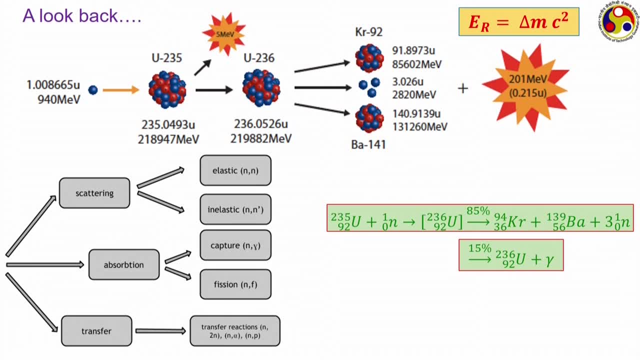 all will happen or not. that strongly depends upon the energy of the neutron and also on the nucleus itself, Like the equation that I have mentioned earlier, that the reaction equation that I am showing here, This particular reaction that is varied only for thermal neutron, that is, the neutron which are having energy of the level of 0.025 electron volt a high. 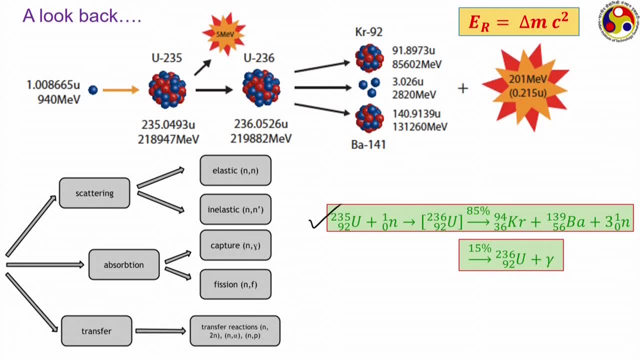 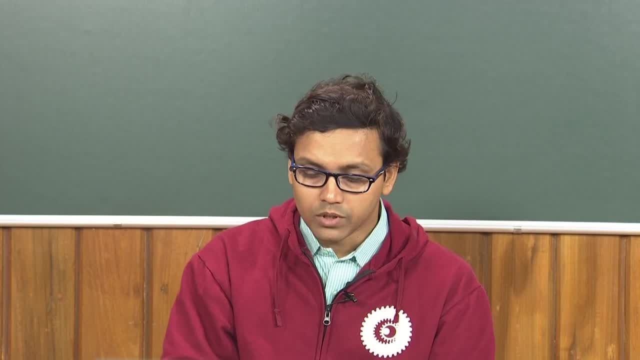 energy neutron generally will not cause such kind of reaction for uranium 235.. So in the fourth module we gave a much closer look to the neutrons, particular distribution of neutrons inside the reactors. We have seen the power produced during reaction can be. given by such a reaction like this, Where the six neutrons, that the energy there is unclear how much is equal to the energy that is making the insertion. last reaction from a certain energy source. However, if all of you only looking at this, 3痛t.1 ReactioneiC. 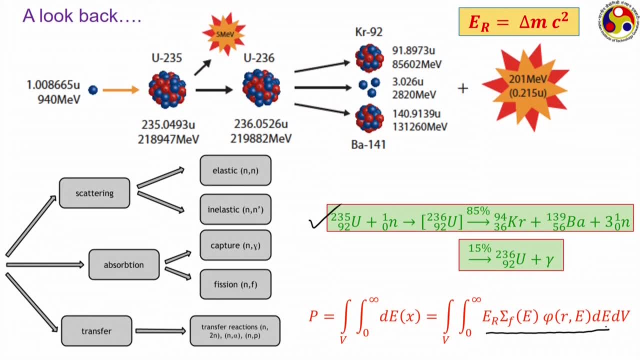 So this particular term isassociated with the amount of energy releasedduring fission. here E? rthis one is the amount of energy released during a single fission reaction, which is generally of the order of 200 MeV. sigma f is a macroscopic cross section, and this is: 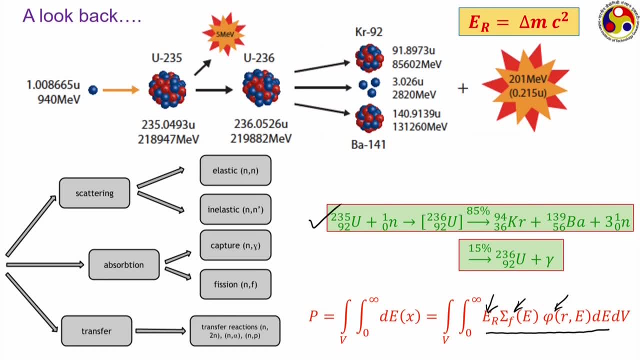 the neutron flask, generally the thermal neutron flux. but here as a neutron can have different neutron can pass through different energy level in reactor, So we need to integrate this over all possible energy levels at any particular location and then to get the total energy produced by the reactor. we need to integrate this over the 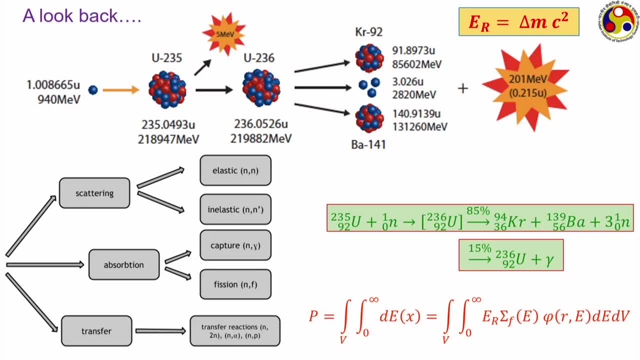 entire volume. Sonow, we more or less know about how to calculate the neutron flux distribution, like we havestudied different cases in the previous module, and once we know the neutron flux distribution, the theknowledge about E, r and sigma f are more or less standard. 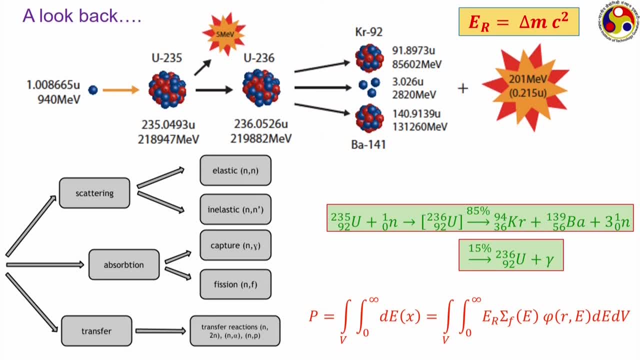 Nowadays, and so just by knowing the neutron flux distribution, we can more or less calculate the total power that has been produced by fission inside a reactor. But once we have the power, and then what to do with that? of course we need to transmit. 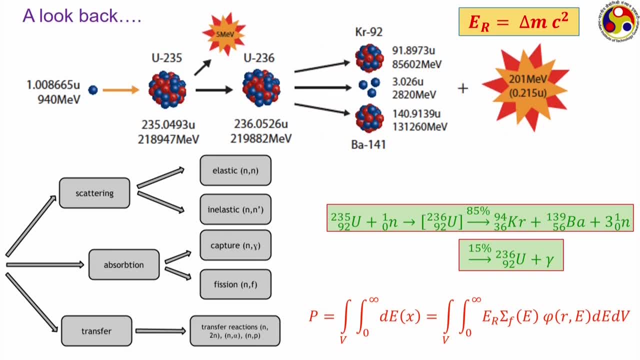 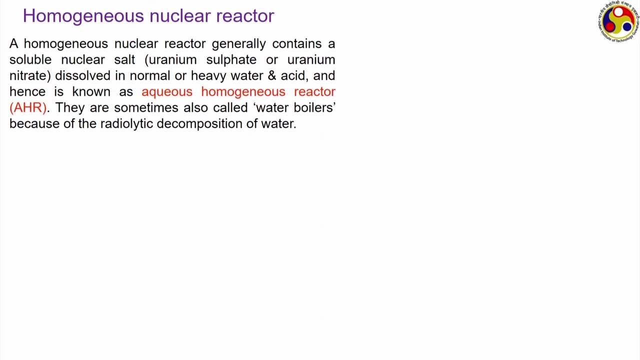 the power to some, some coolant stream which will be used for subsequent power production, and in this particular module we are going to look at that particular power transmission or energy transmission procedure. Now, to start with, I probably have mentioned earlier that commonly we can classify nuclear 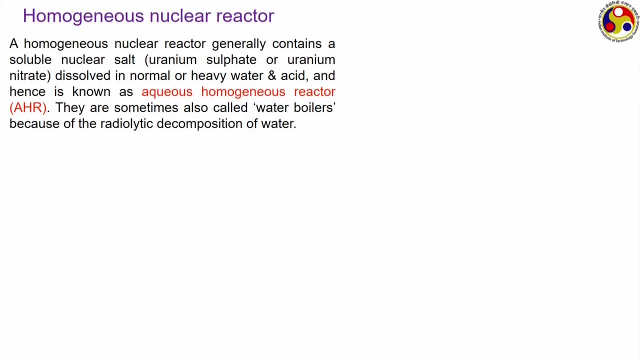 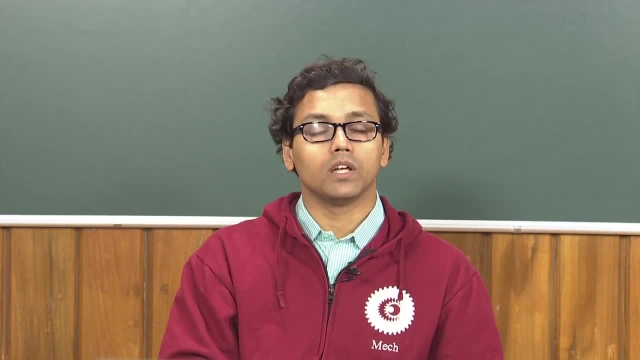 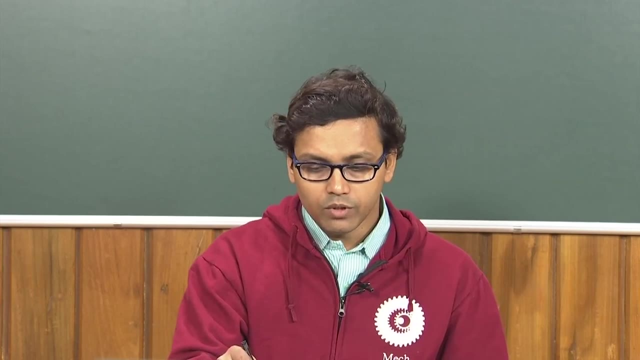 reactors into two categories: homogeneous and heterogeneous. A homogeneous, nuclear refers to the one where we have an uniform distribution of all the substance that may be present inside the reactor, That is, from the entire volume of the reactor. let us saythis is one reactor. Now, if we pick up a sample from somewhere here and a sample from somewhere here and 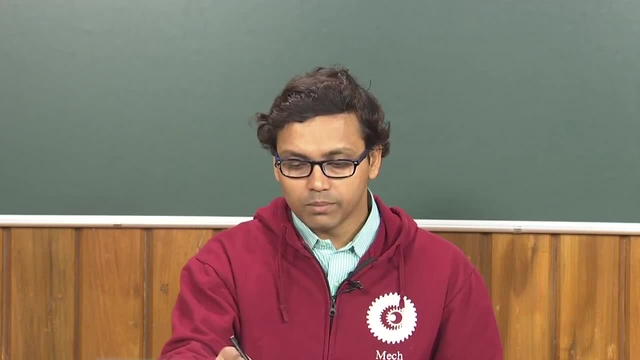 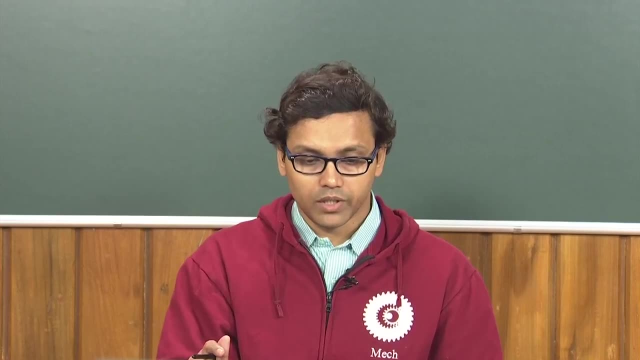 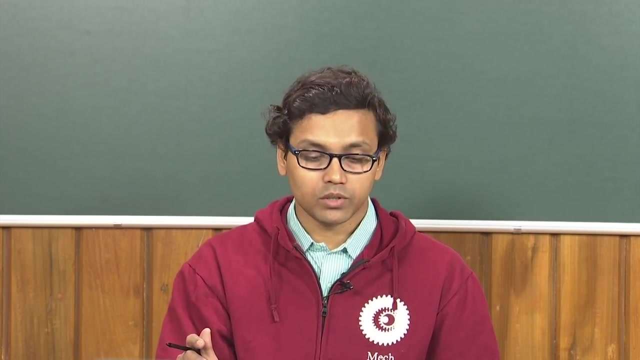 a third sample from somewhere here, And all these samples should have identical chemical composition, and then only we shall be calling it a homogeneous nuclear reactor. Generally in a homogeneous reactor we have a soluble nuclear salt, commonly sulfate or nitrate salts of uranium, which is dissolved in water. 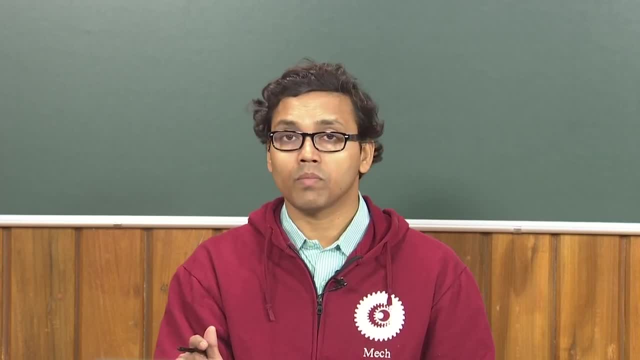 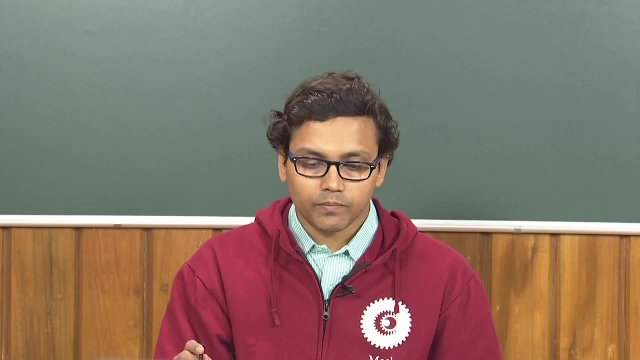 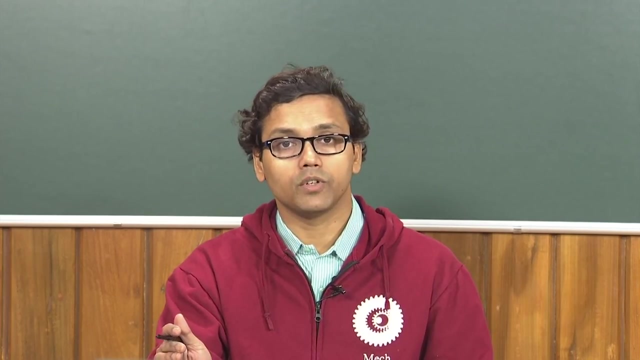 Now that water can be the normal water or it can be heavy water also. just remember that heavy water refers to the water where hydrogen is actually deuterium. Now, here the nuclear salt is generally dissolved in normal heavy water, and also acid, as it can be sulfuric or nitric acids. 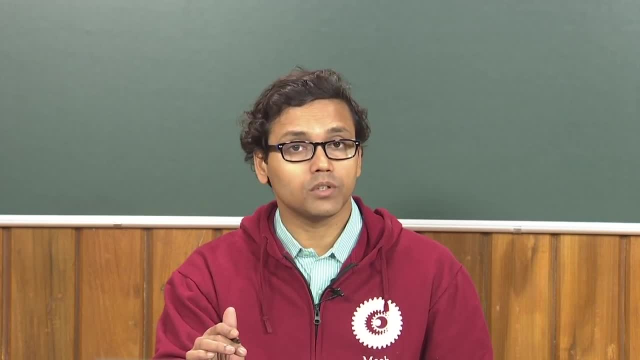 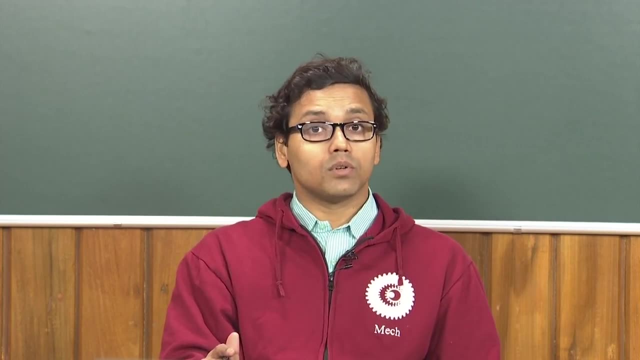 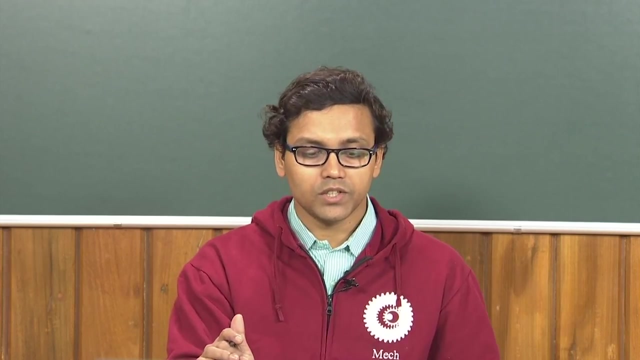 And this kind of say because of the presence of such an aqueous solution of nuclear fuel. there are also called aqueous homogeneous reactor, AHR There also sometimes called water boilers. do not get confused with boiling water reactor, which is a common type of nuclear reactor. water boiler refers to this, AHRs. 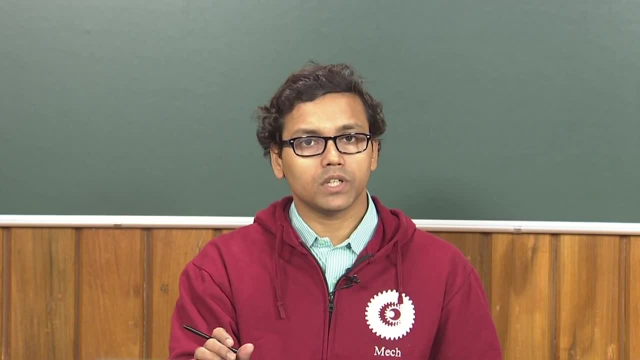 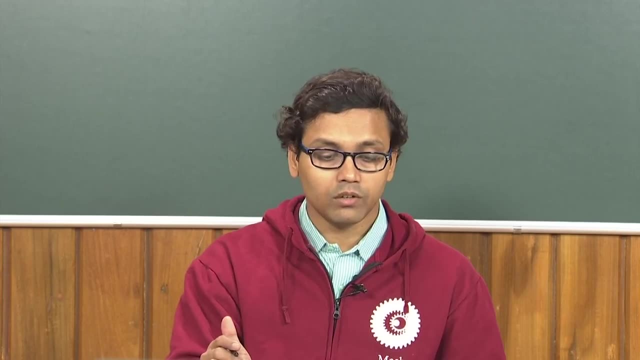 molecules that can be present inside the reactor. they can go through a kind of a decomposition process when that is subjected to the radiation, Such kind of radiolytic. because of such kind of radiolytic decomposition, hydrogen and oxygen bubbles may appear inside this reactor. 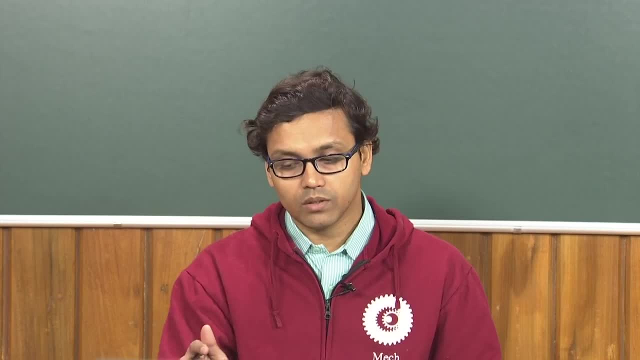 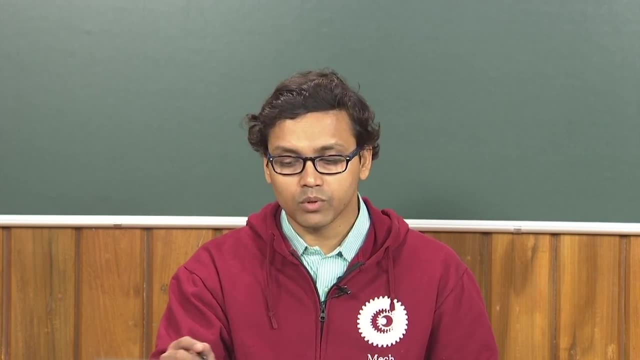 and that is why they are called water boilers. This is a classical picture of a very old and popular AHR developed in the Oak Ridge National Laboratory. We do not want to go to the details of this, just for your idea, where we have a common vessel and inside the 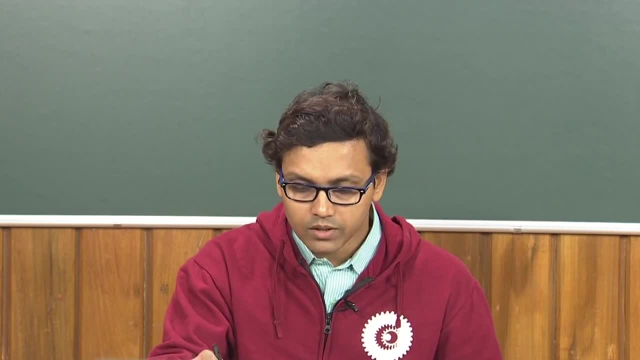 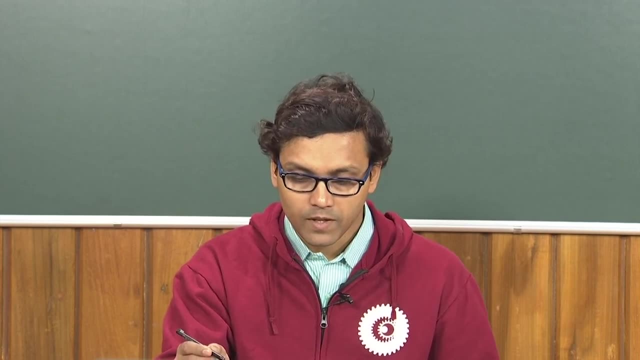 vessel. inside this pressure vessel, like this one, inside this pressure vessels, we have this aqueous solution of the nuclear fuel and everything takes place inside that. You can see it is a 60 inch diameter, which is a very large one. Now, homogeneous nuclear 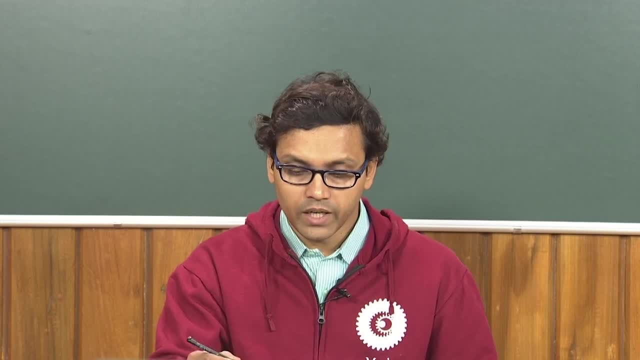 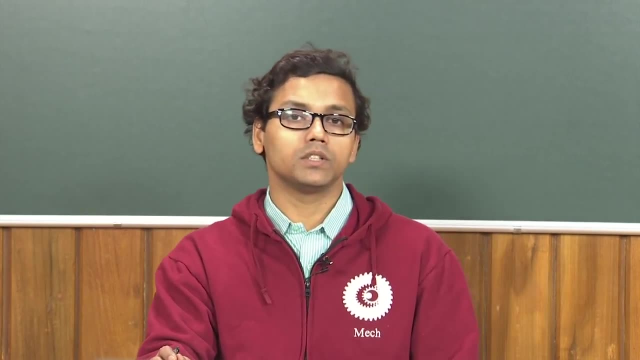 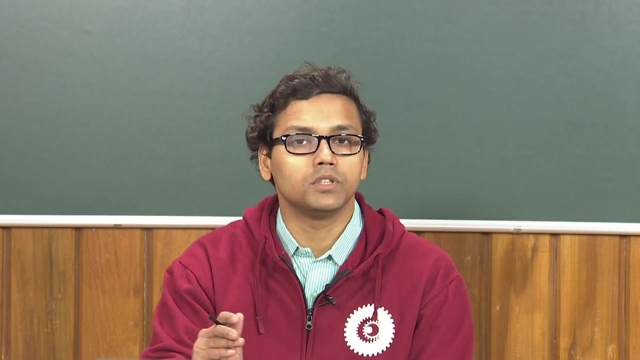 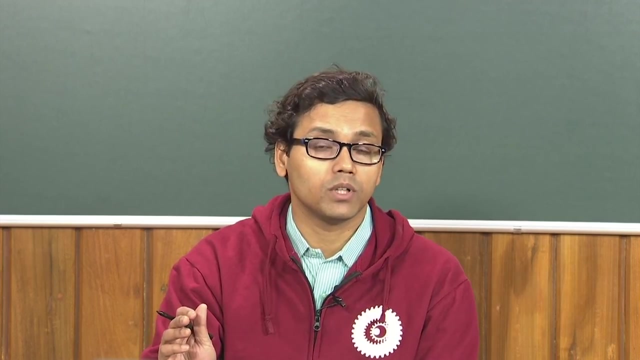 reactor offers several advantages, like it can attain criticality with the natural uranium itself. If you think about the earlier analysis of multiplication factor that we have done, to have a criticality condition we need to have a large value of this thermal fission factor and also significantly large value of the thermal utilization factor- Now a natural 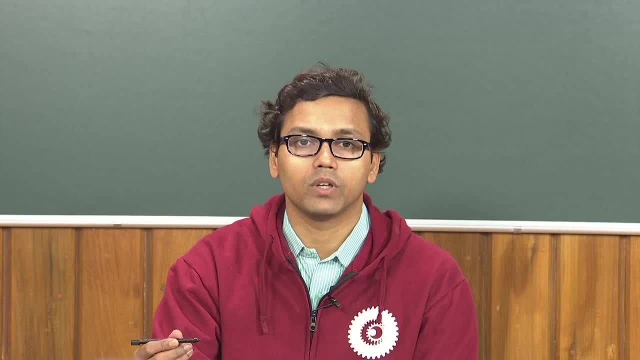 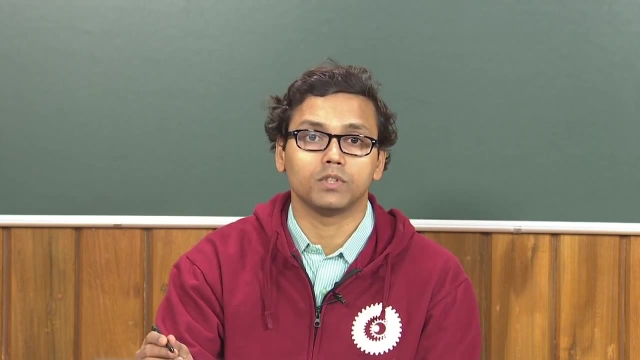 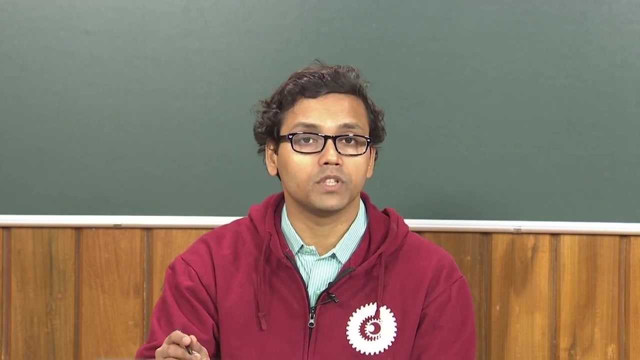 uranium has only 0.7 percent of uranium 235, rest is uranium 238. Therefore it can have quite significant value of this resonance factor, This resonance absorption probability, but still because of the large volume and uniform mix, a large volume of the shell and uniform mixing of fuel and moderator, the homogeneous. nuclear reactor generally can attain criticality with natural uranium itself And quite frequently they are also used with enriched uranium. and if they are used in enriched uranium they provide an excellent specific fuel requirement which is generally very low compared to other kind of reactors. that is heterogeneous nuclear reactors. 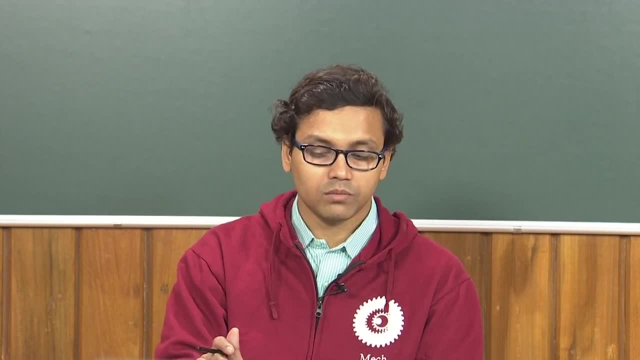 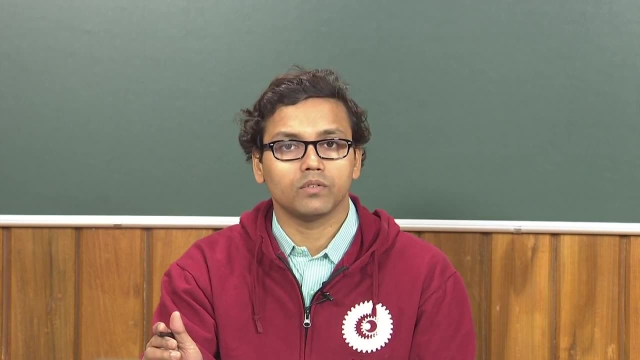 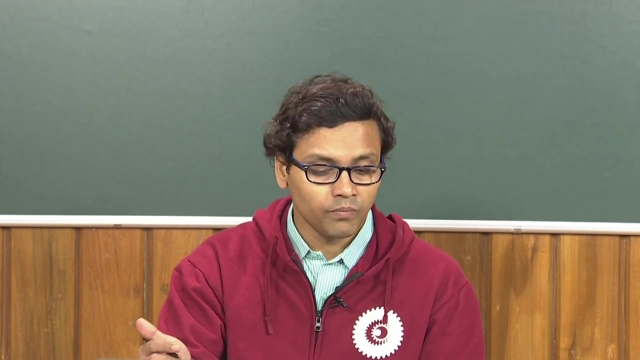 Neutron economy is also superior in case of homogeneous version, because the neutrons are surrounded by neutrons and fuels on all the sides And therefore, that is, every neutron is surrounded either by moderator nuclei, moderator nuclei or fuel nuclei, And therefore there 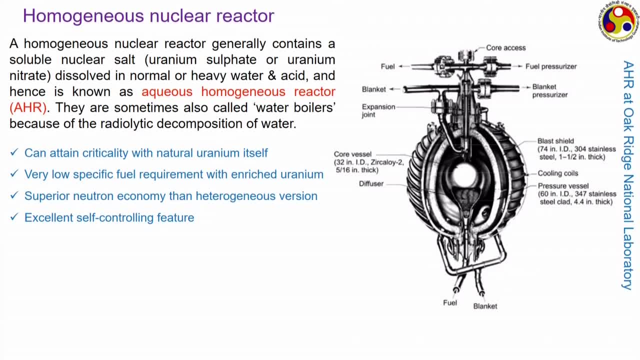 is excellent neutron economy compared to heterogeneous version. They are also very good in self controlling and can handle large increase in radioactivity because of their large volume of moderator and coolant present cells. However, homogeneous nuclear reactors are not very popular for commercial use because of their challenging kinetics and control. 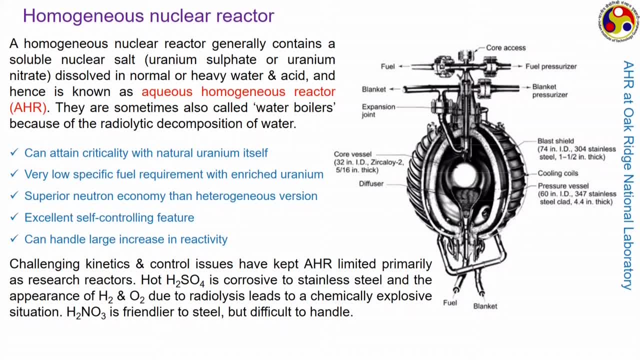 issues. While they have very good self controlling feature, the external control is quite difficult, again because of that homogeneous mixing only. we cannot independently control the reactivity. yes, ah, because once we get the reactor started We do not have active reactance reaction, So we cannot control reactivity and result. 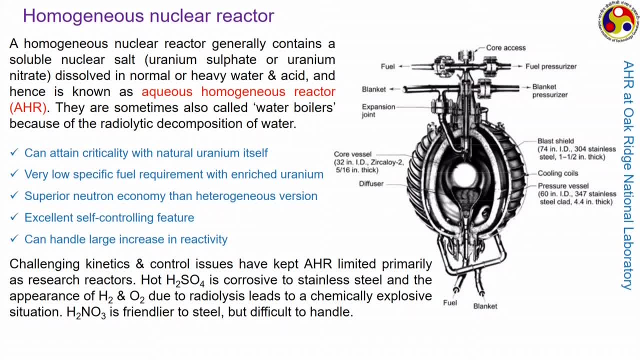 exclusive control on the mass of fuel and the mass of moderator that is present there and also we do not have means a direct control on their on the reactivity. So AHR is primarily limited to research reactors: lab scale, small reactors, till date A big 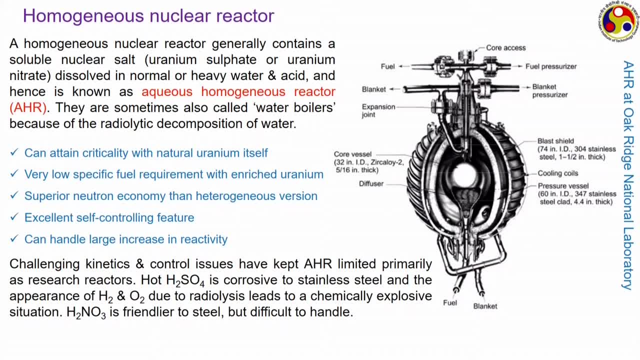 problem for them is also the use of the sulphate or sulphuric acid. Urine and sulphate in water leads to the production of sulphuric acid, and such hot sulphuric acid is extremely corrosive to stainless steel, which is one of the common materials used in nuclear reactors, And also 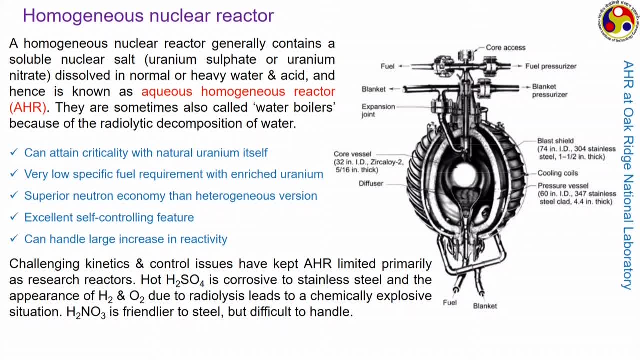 the appearance of hydrogen and oxygen bubbles because of the radiolitic decomposition is another big issue from control point of view. When we are using the uranium nitrate as the fuel, then we do not have sulphuric acid, rather we have hot nitric acid. Nitric acid is much. 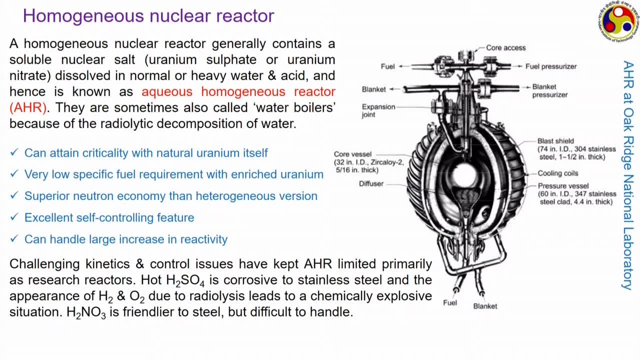 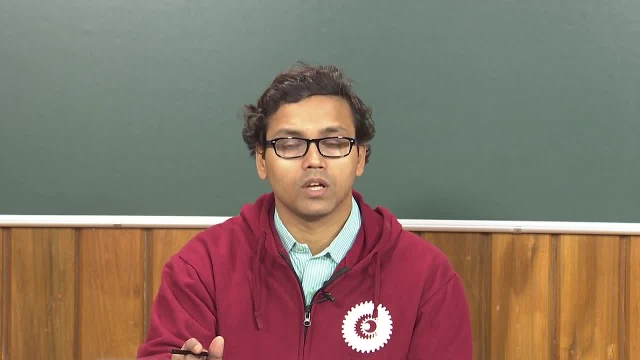 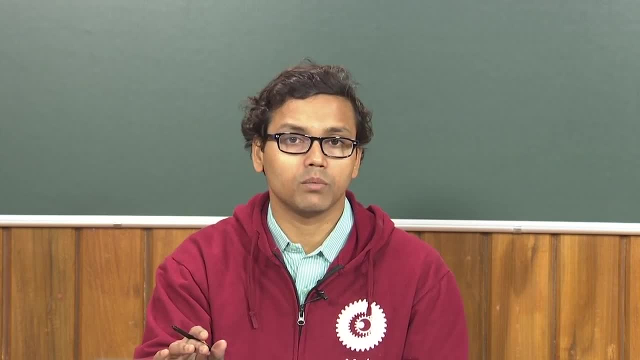 friendlier to stainless steel, That is, it does not corrode stainless steel that much. but everyone knows how difficult it can be to handle nitric acid, particularly at higher temperature. So these are the reasons of not using homogenous nuclear reactors. that much for commercial power generation Rather. 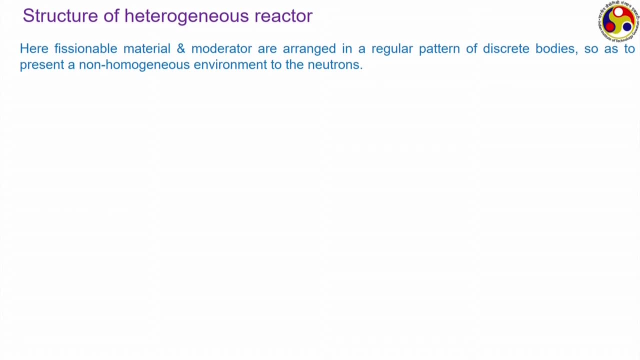 for new commercial power generation In heterogeneous nuclear reactor we have material, the fissionable material, that is a fuel, and moderator keeps separately, But they generally arranged in some kind of regular pattern, some kind of repeatable regular pattern, And every fuel component is generally separated by moderator with the adjacent fuel components. 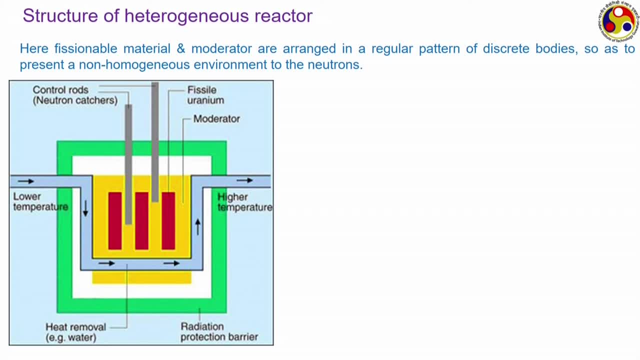 Just represent a picture like this. here the red blocks are actually fuel, which are surrounded by moderator, this yellow colored one- from all possible sides The coolant is flowing. this blue line refers to coolant through which which is flowing through the reactor core and therefore all the energy that has been generated, because 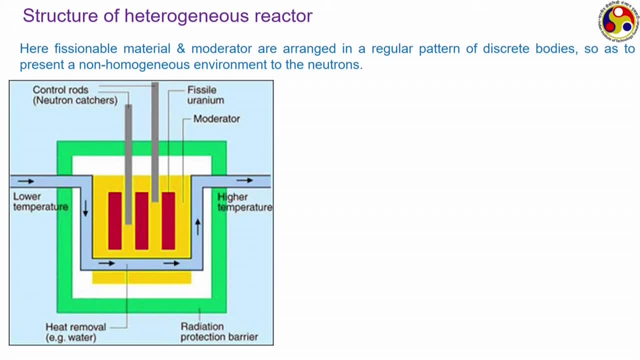 of the fission reaction that are taken by this coolant stream. We can also have the control rods, which are one of the controlling units, which will discussing them in the next module. This is just a representative picture, but this red blocks of fuels that we can find. 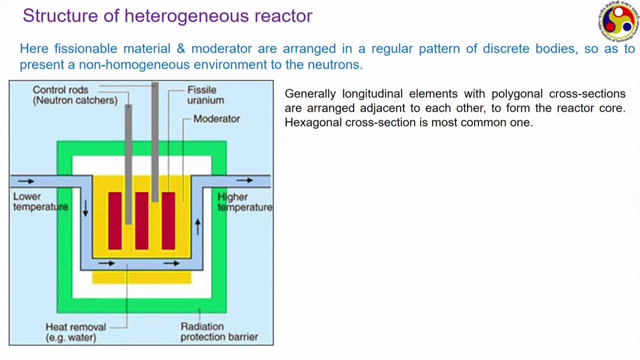 in practical cases also, they look more or less the same. We generally can have two types of designs. one: we can have plate type of reactors that is not reactor, I should say plate types of fuel elements, Where every fuel element is shaped like a rectangular plate, very thin rectangular plate. 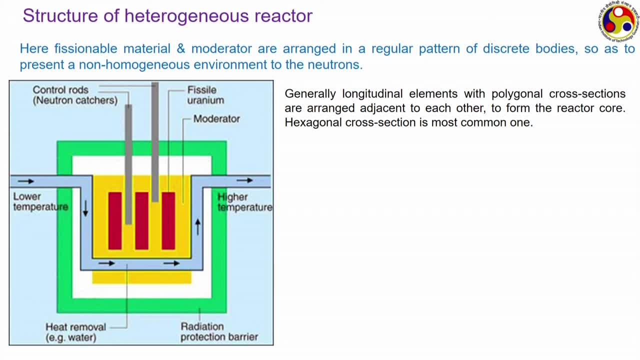 I should say, and then immerse into moderator. Other possible design can be of circular cross section, cylindrical design. again, the diameter of the cylinder generally is kept quite small compared to its height. There are generally longitudinal elements with polygonal cross sections which are arranged adjacent to each other. 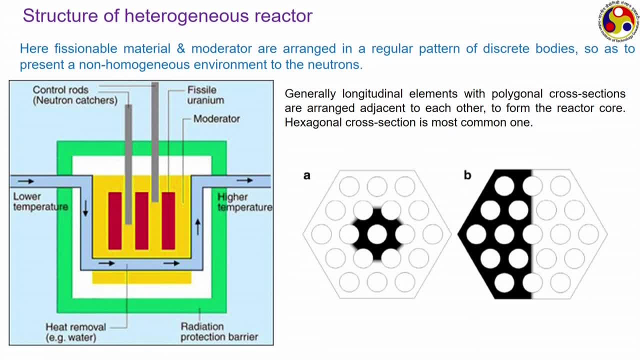 Hexagonal cross section is the most common one, Just like shown here. all the circular elements are the fuel rods. cylindrical fuel elements are called fuel rods, The circles are fuel rods and all the gaps in betweens are occupied by moderator or the coolant. 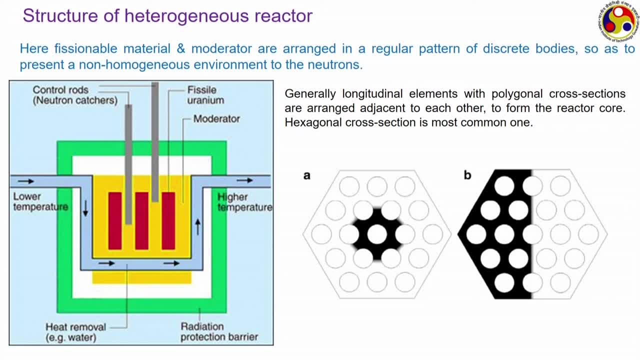 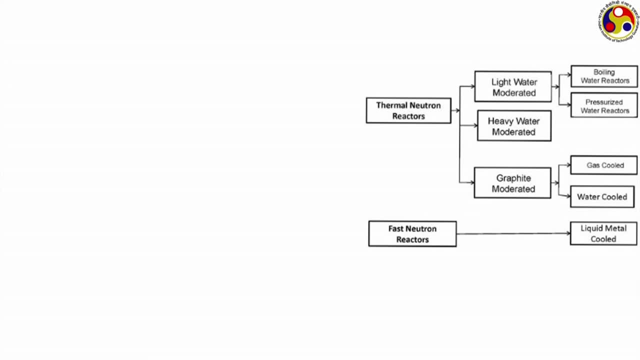 We can also have rectangular or triangular cross sections in nuclear reactors, but hexagonal is mostly preferred. Now, nuclear reactors can be classified into different categories as well. Actually, from now onwards, we are not going to use the term heterogeneous, because we are going to talk only about heterogeneous. 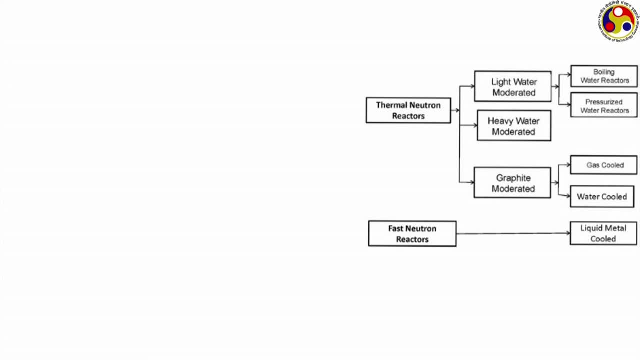 We are going to talk about heterogeneous nuclear reactors, and heterogeneous reactors can have several kinds of classification, like one class. common classification is based upon the neutrons that are being used inside. So based upon the neutron flux profile, we can have first neutron reactors or first reactors. 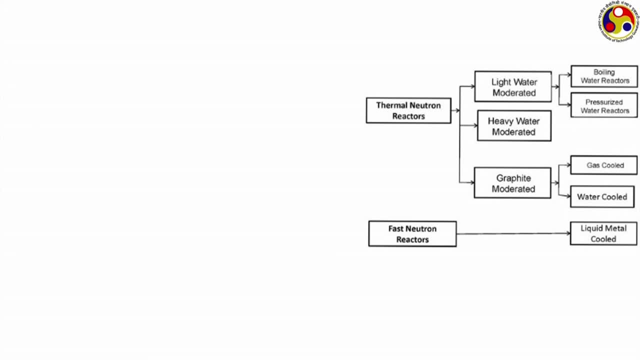 and thermal neutron reactors, or thermal reactors. Fast neutron reactors, of course, utilizes fast neutrons for their operation, and hence they must use a fuel which has some significant value of this fast fission cross section. The next one is NPPD. This is the class of carbon fiber. 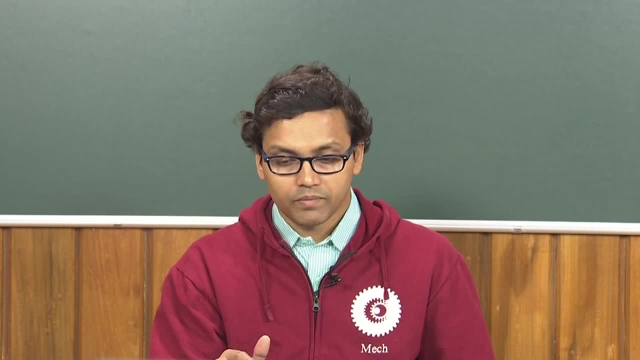 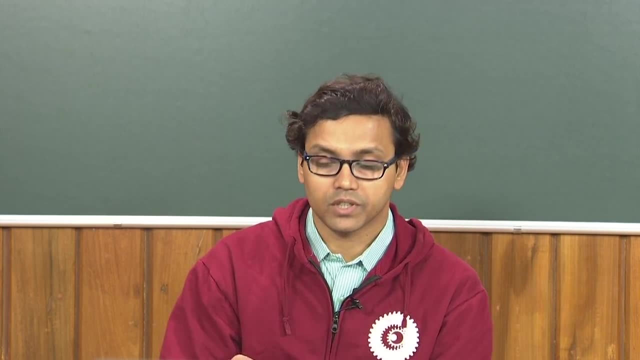 This is the class of carbon fiber section. Similarly, ah thermal neutron reactors utilize thermalized neutrons, So there is a big role of moderator in case of thermal reactors. based upon moderator, thermal reactors can be classified as the light water moderated reactor, heavy 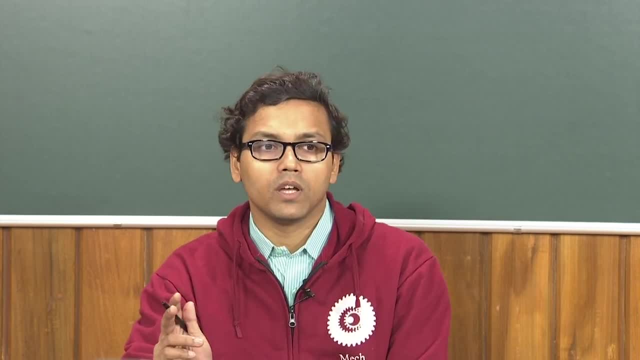 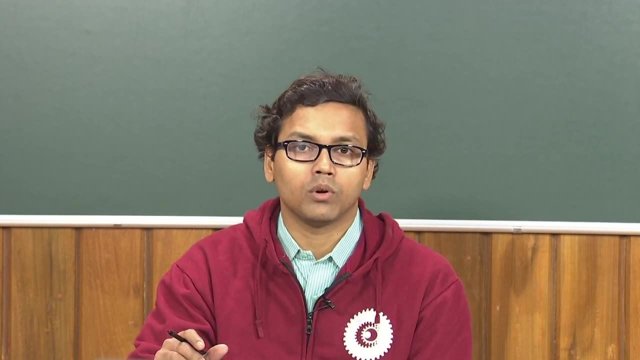 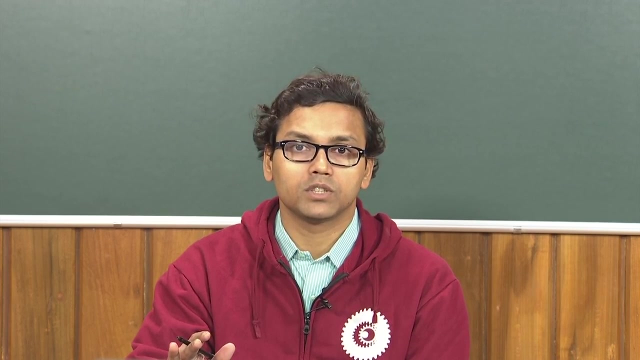 water moderated reactor and graphite moderated reactor. Here I would like to mention again that light water generally is a quite bad term because it here we are talking not about any water which is lighter than the common fluid, rather we are talking about the common water itself. but still, just to differentiate them with heavy water, this term is universally. 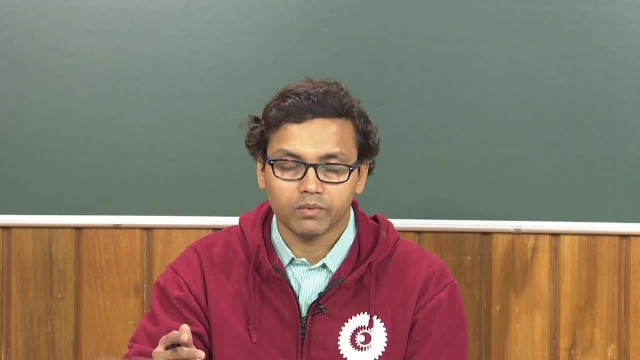 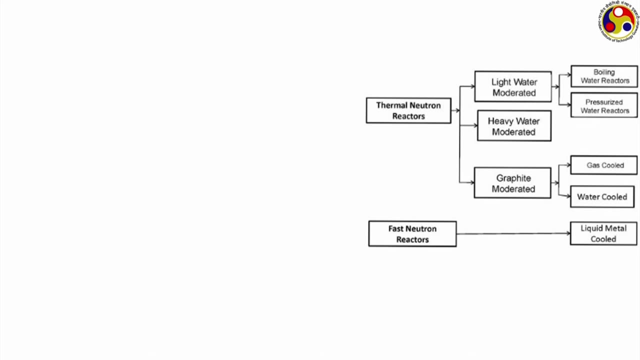 used in the case of a nuclear field and therefore at least in this kind of names we have to use this light water reactor kind of terminologies. Now there can be three kinds of moderators, like normal water, heavy water and graphite and this light water, so called light water. 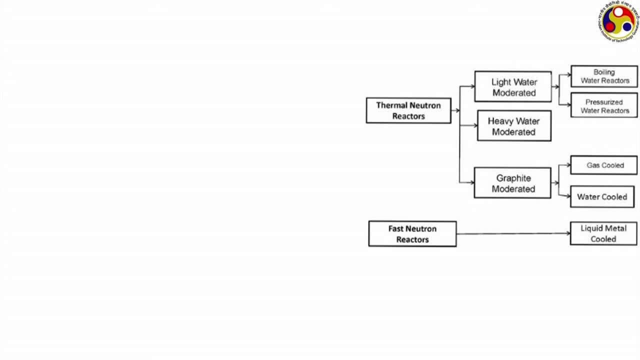 reactors again, can have two principles, Four principal classifications: boiling water reactor and pressurized water reactor. There can be quite a few others also. we shall be talking about them later on. Similarly, graphite moderator reactors also, depending upon the nature of the coolant, they can be a gas cooled. 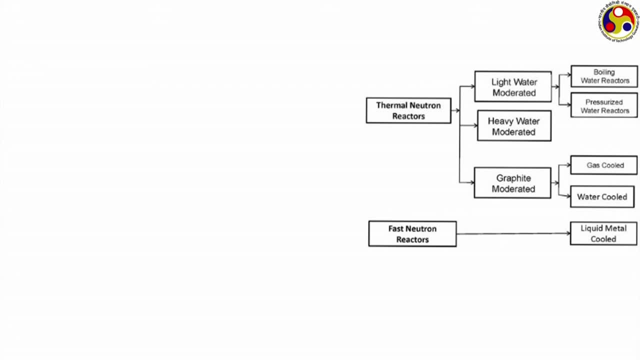 or water cooled and in case of fast neutron reactors, what can be the moderator in a fast neutron reactor? What is the purpose of moderator? The purpose of moderator is just to slow down a fast neutrons to the thermal neutron level and in a fast reactor we are looking to utilize. 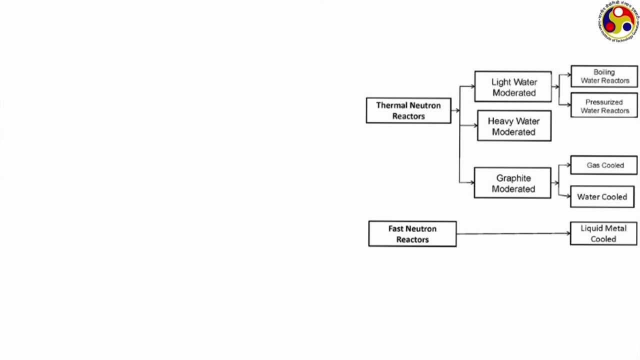 the fast neutrons. So to slow down a fast neutrons to the thermal neutron level, So neutron itself or we, and we are not at all trying to slow it down. And therefore a fast neutron reactor does not have any moderator, rather it the fast neutron itself induce fission. 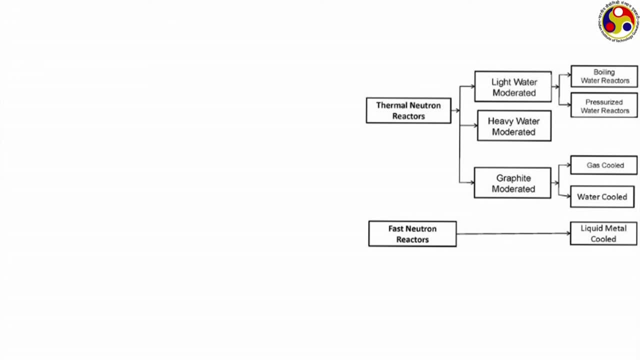 to the fuel and transfer that energy to the coolant. Fast neutron reactors are generally liquid metal cooled, that is, they use liquid metals as the coolant name. This is a common schematic diagram for a pressurized water reactor. In case of a pressurized water, 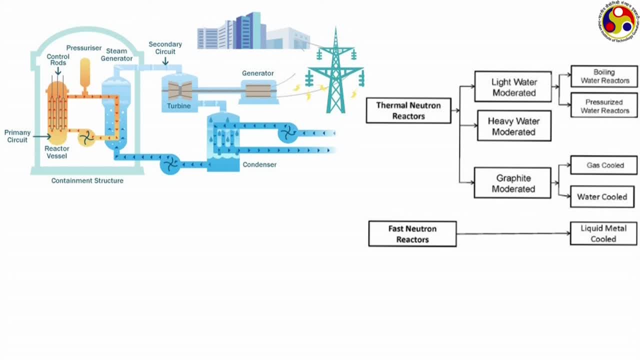 reactor, the water is maintained in single phase by using a pressurizer. The pressurizer maintains a pressure inside the reactor such that that maximum temperature of water is not allowed to cross the saturation temperature, And hence we are having single phase operation. And this is a boiling water reactor. in case of a boiling water reactor, the water or the 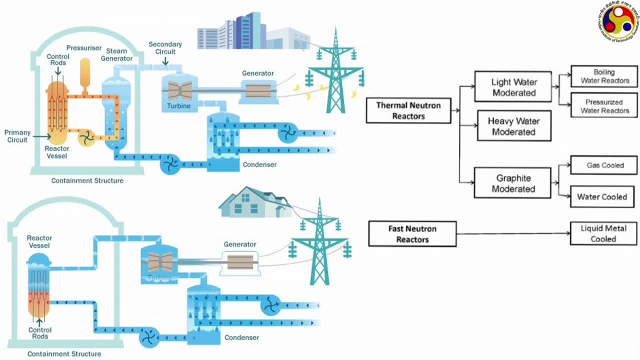 fluid is allowed to boil and gets converted to steam, or I should say a part of that water gets converted To steam and the steam is taken through the subsequent processing in the form of turbine and expansion in the turbine and condenser and pump, and again back to the core in the 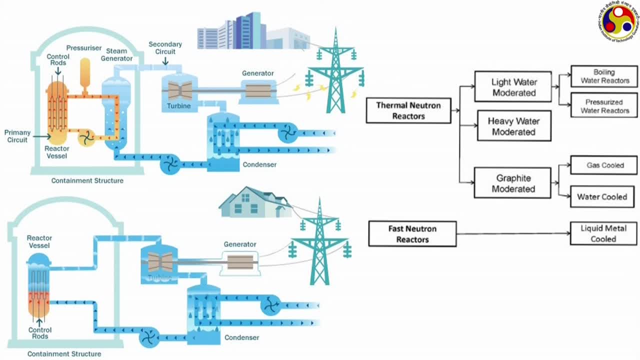 form of recirculation So we can have wide variety of coolant. as we can see from here, These two, both these two figures- refers to light water reactors. but in one case we are using single phase water to carry all the heat, So we carry all the heat produced by nuclear fission, whereas in the other case we are using 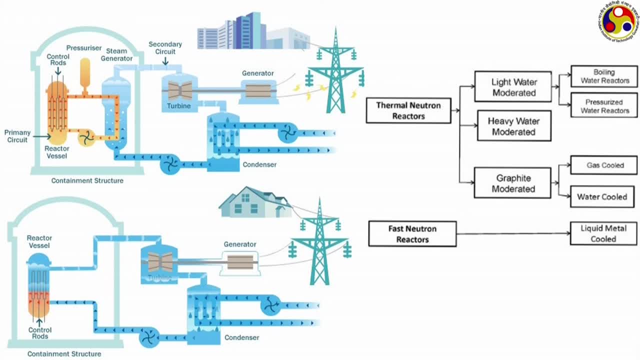 the phase change process to carry the heat from the nuclear reactor. We can also have gas cooled reactors which, again quite similar to the pressurized water reactor. they remain in single phase, single phase gaseous medium, but their gas is allowed to circulate through. 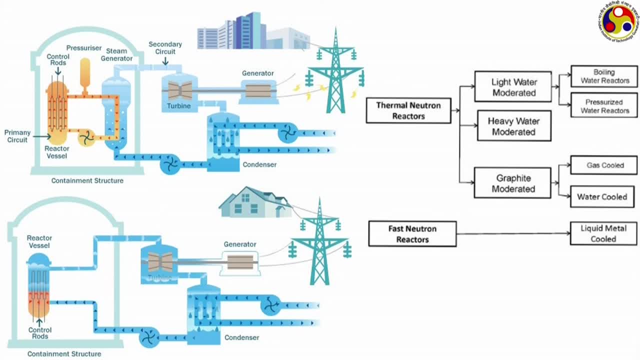 the core and transfer the heat to subsequent downstream operation and then come back again. Same about liquid cooling. 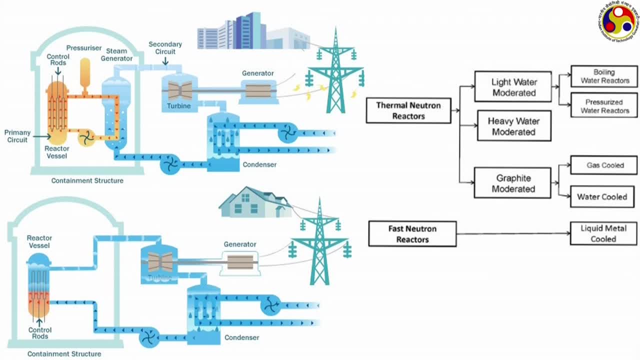 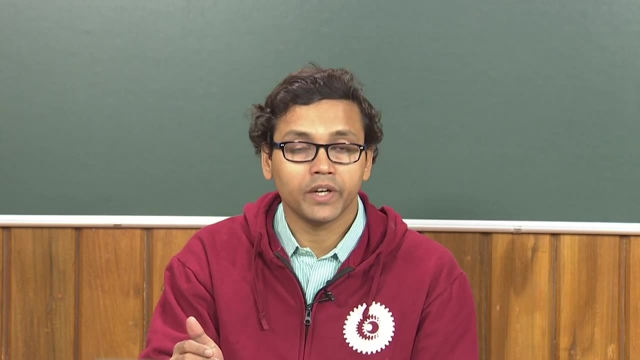 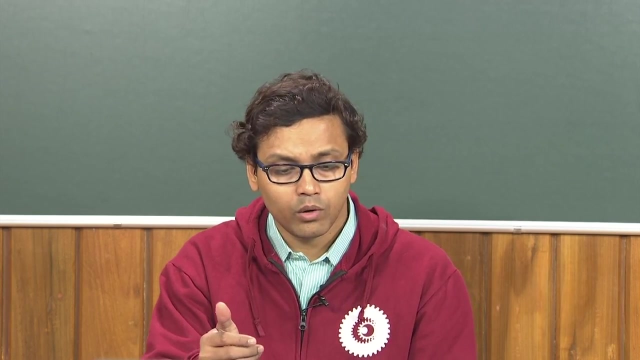 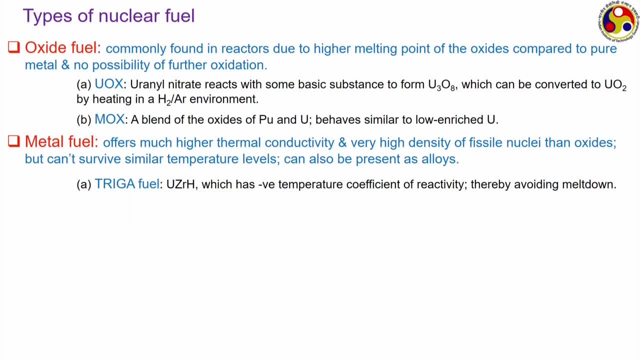 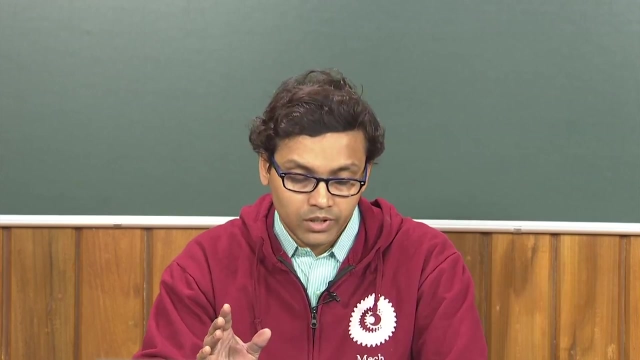 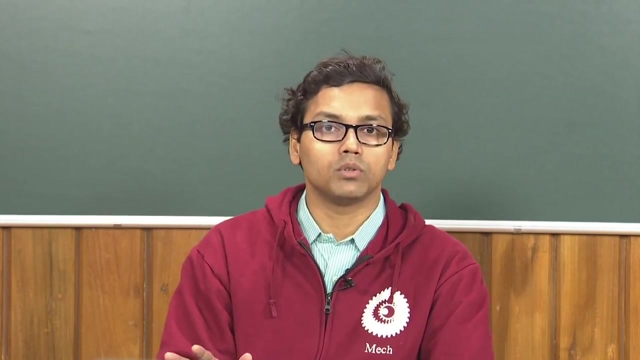 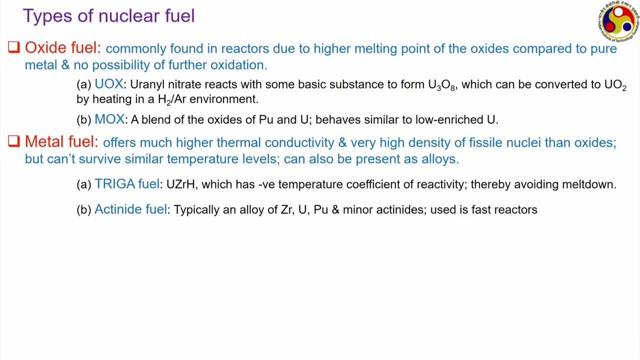 There can be ceramic fuels as well. Ceramic offers um very high thermal conductivity and melting point, but they are prone to neutron induced swelling that is at higher temperature. 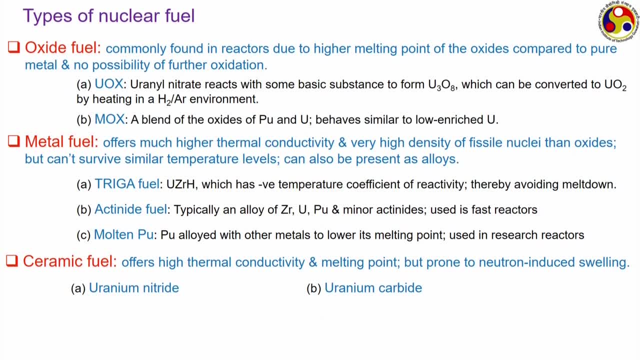 there may be a significant change in his volume. hm. there we can have commonly uranium nitride and uranium carbide as the 2 ceramic foils. and the final category is that of the liquid fuels. Liquid fuels are generally using the homogeneous reactors and not that much in heterogeneous reactors, for obvious reasons. Liquid fuels- 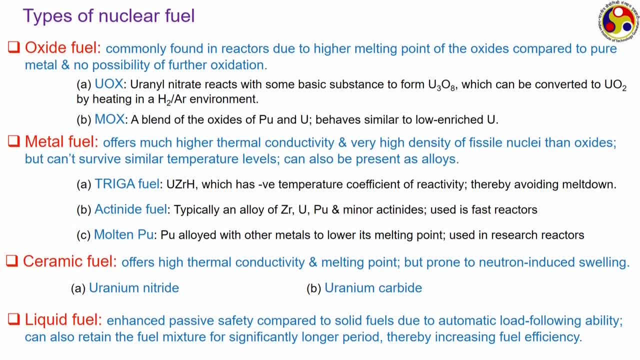 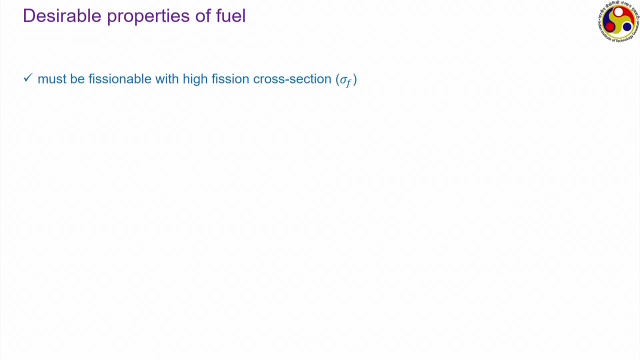 enhances the passive safety compared to solid fuels. because of automatic load following capability, like we have in case of homogenous reactor, They can also retain the fuel mixture for significantly longer period, thereby affecting the fuel efficiency. So, with all these kinds of fuels in any reactor, while choosing the fuel we can consider several. 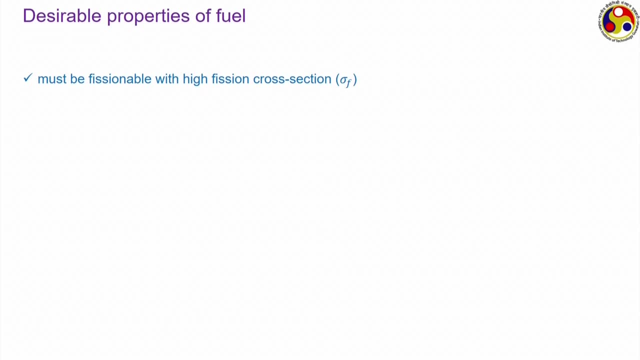 factors like the fuel must have a very high fission cross section. Secondly, it should have a very high thermal conductivity. If the thermal conductivity of the fuel is high, then the temperature change across the fuel itself will be will be quite small. These are common values of thermal conductivity. like for metallic uranium thermal conductivity. 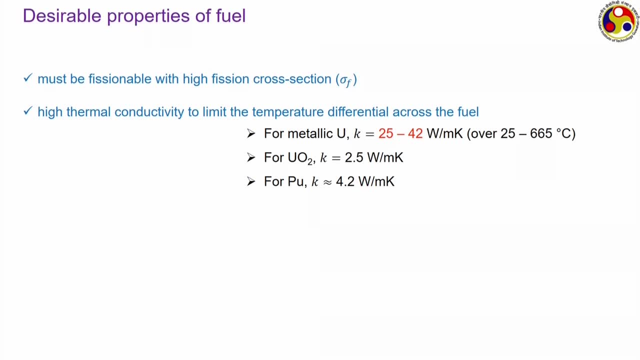 may vary between 25 at 25 degree Celsius to 42 watt per meter Kelvin at 665 degree Celsius. For uranium oxide it is much higher than the much lower just of 2.5 watt per meter Kelvin, Whereas for plutonium also has a conductivity. 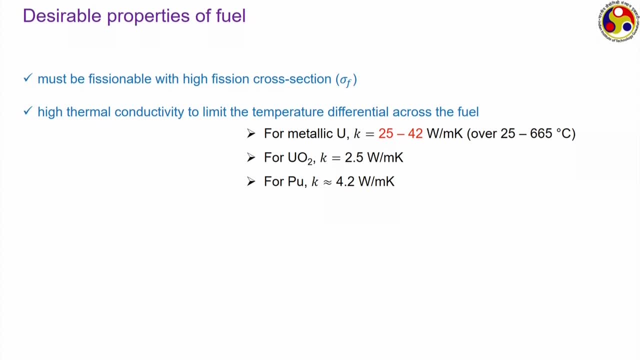 lower than uranium, which is something like 4.2 watt per meter Kelvin. The at higher temperature. the fuel should have sufficient mechanical strength so that it can maintain its own shape and does not get deformed. ah, Like uranium, is unusable beta beyond 665 degree. 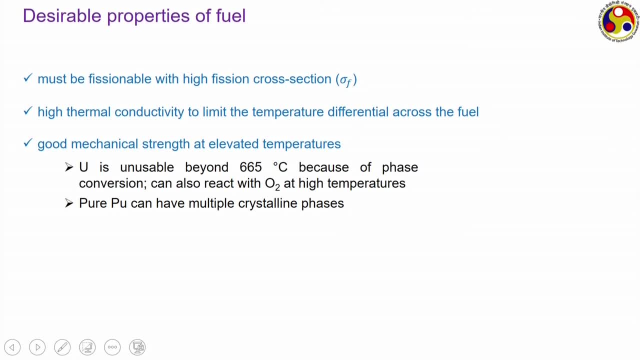 Celsius, because uranium can have several crystalline phases, like alpha, beta and gamma phases, and beyond 665 degree Celsius. So that means the translation from alpha phase to the beta phase. Uranium can also react with oxygen at high temperatures and get oxidized. And another problem with plutonium. 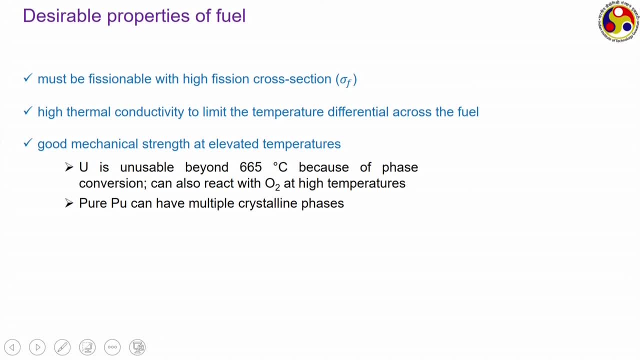 is pure fuel is. it also has several crystalline phases And therefore not suggested to be used at high temperatures, or at least high core temperatures. The temperature range available for operation should also be large, and that is possible only when the solid fuel has a high melting point. Now the next big point, which is the thermal conductivity we 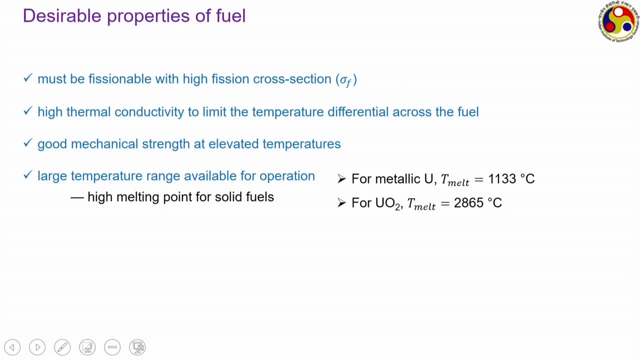 melting point. like for pure metallic uranium, the melting point is something like 1133 degree Celsius, whereas for uranium oxide it is significantly higher. it is greater than 2800 degree Celsius. That is one of the reason of not using metallic uranium, rather uranium oxide, as the fuel in 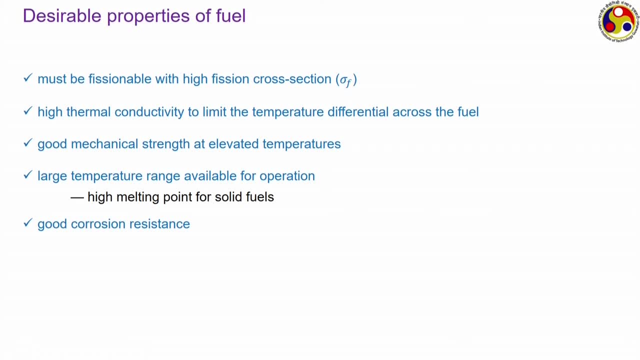 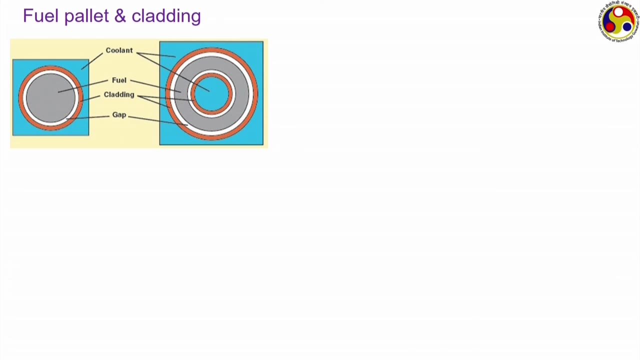 modern reactors. And finally, they should also have good corrosion resistance characteristics, because they generally remain in contact with flowing coolant, which can cause- or try at least can try to cause- significant amount of corrosion. Then we come to fuel pellet and fuel cladding. Pellet refers to its small module of fuel. 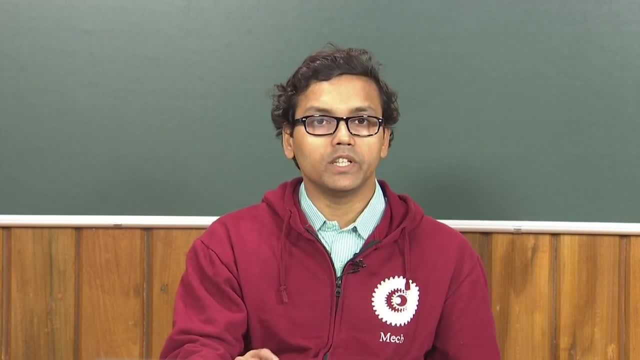 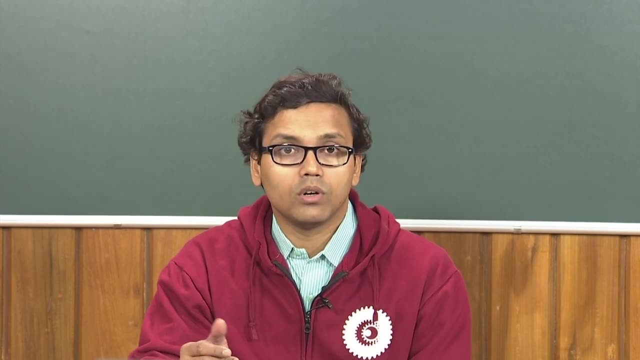 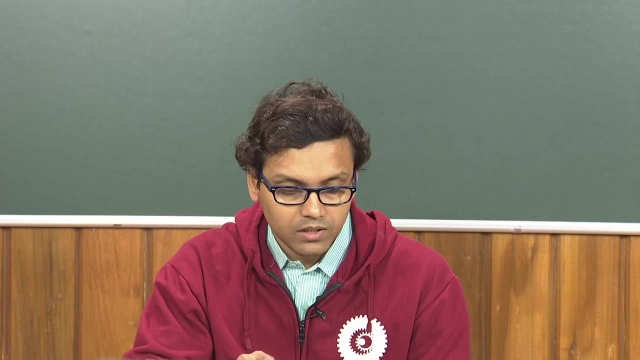 element which can be of the shape of small bullets or maybe a just like a small tablet, and they are covered by a jacket which is called cladding. Claddings have several important purpose Because like this is a much elaborated diagram where you can clearly see each of the fuel. 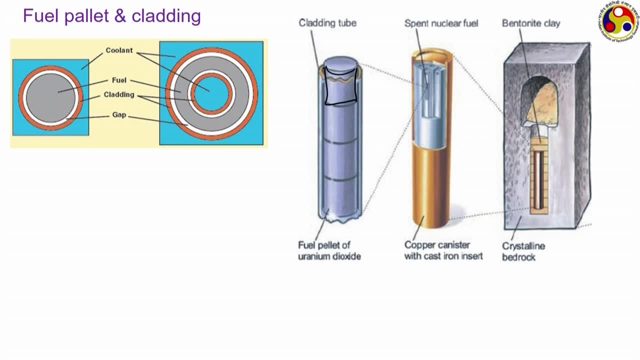 modules here like this is the one. this one is a fuel module and this module is being covered by the cladding material. So some, several fuel modules, each one is put on top of the other one and they are connected from energy point of view and their cladding is. 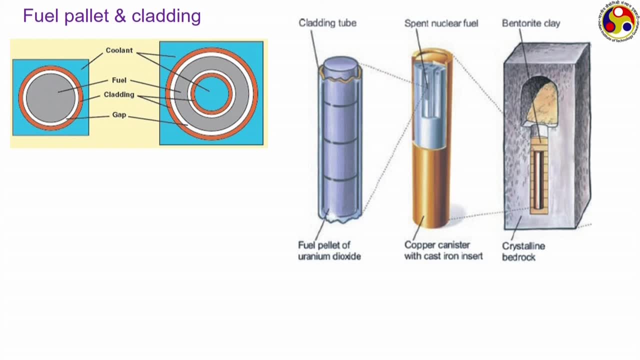 also a common material and hence the cladding must have can serve several important, important functions, like they can provide the structural support to the fuel and thereby prevent distortion. That means at higher temperature, even if the fuel gets soften or become soft, then it will. it cannot go just directly into the coolant stream, rather they would remain inside this. 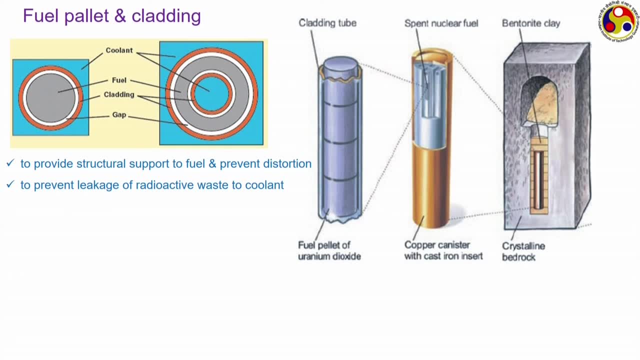 cladding tumble. Another advantage is to prevent leakage of radioactive waste to coolant- The radioactive wastes that are being produced. that generally remains inside the reactor itself. It is later on. they can be means. once their lifetime finishes, they can be used as this spent fuel. And finally, 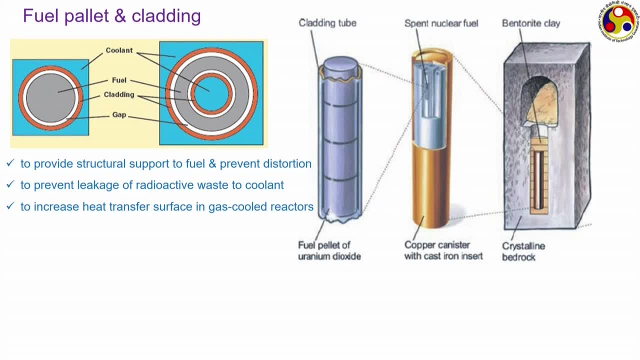 this, so radioactive leakage of this waste to the coolant can be avoided. And finally, the same positive factor is evaluation of thermal conductivity should be observed. This wszystkie activity is accompanied with 매交通, ygenedic pensions, as assured by heat transfer coefficient. 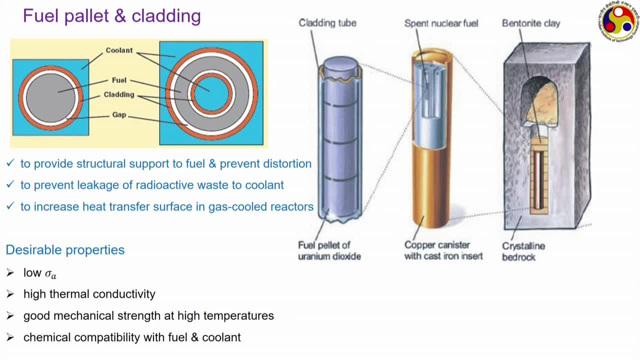 This cladding some kind of complex heat transfer across This cladding? by properly designing the client tube we can. we can also enhance the heat transfer in case of a gas pooled reactor, whatever energy the cladding receives from the fuel that is able to transmit that immediately. 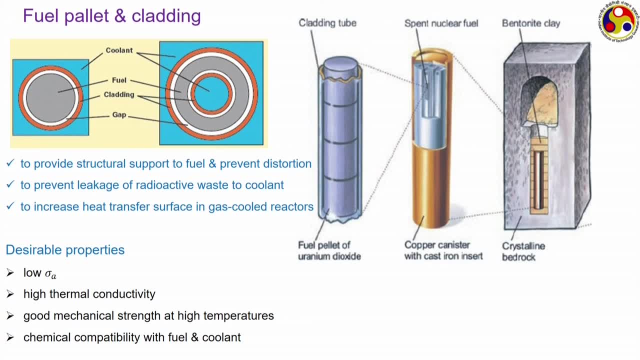 to the coolant. The first point I must go back: low absorption cross section, ah, we have to ensure, because if the cladding itself is starts absorbing neutron, then that will be a type of loss. Then it should have good mechanical strength at high temperature so that you can support the fuel itself. and finally, cladding material. 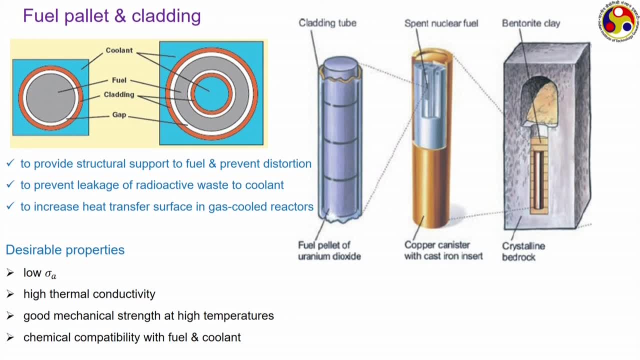 should have chemical compatibility with the fuel and the coolant, particularly the fuel. This fuel, cladding and coolant- all these three materials generally are ah generally, must have compatibility with each other, and so is the moderator. These are the common cladding materials. like aluminum, ah is can be used only for temperatures ah less than. 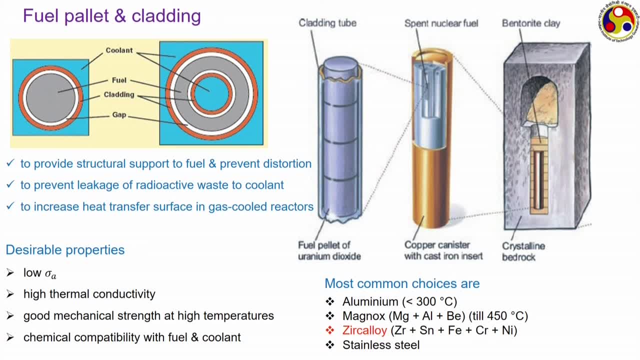 300 degree Celsius and ah, ah. the second very important cladding material can be Magnox, which is actually Aluminum. It is a alloy of magnesium and it can have aluminum and barium along with magnesium in it, and it can sustain up to a higher temperature of 450 degree Celsius. Third one, there is. 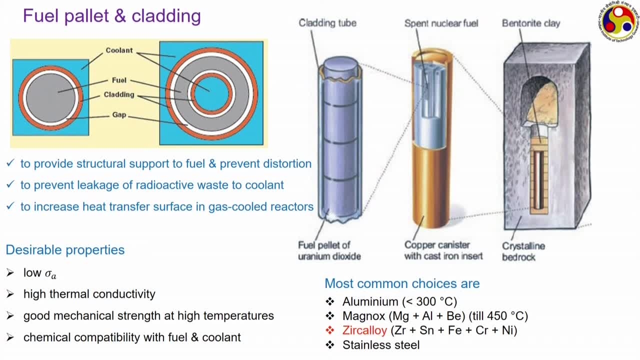 the most preferred one: Zirc alloy, which is an alloy of zirconium and contains small elements like tin, iron, chromium, nickel, etcetera. And finally, stainless steel can also be used, But stainless steel can also be used. But stainless steel can also be used. 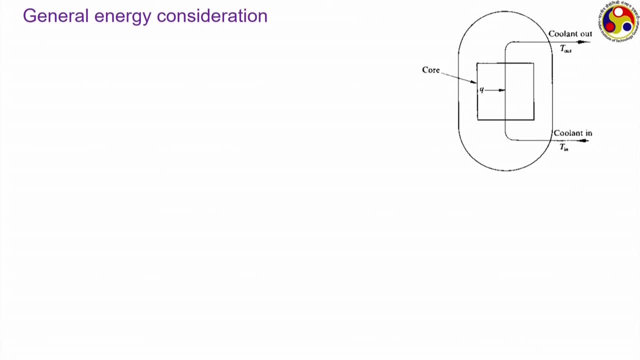 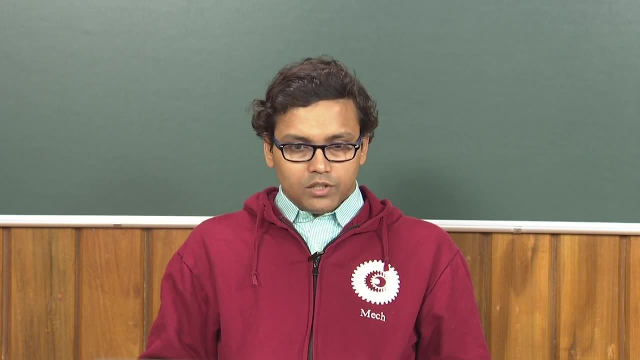 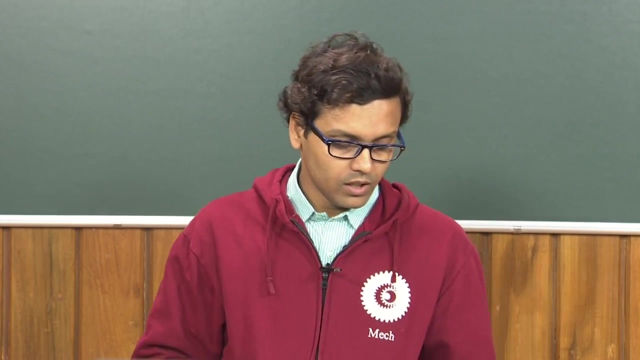 stainless steel may have its own issues. So once we know about the structure of the fuel, we are now ready to study the energy analysis or perform an energy analysis of a reactor, or maybe just a single fuel element. We know that every fuel is covered by a jacket. 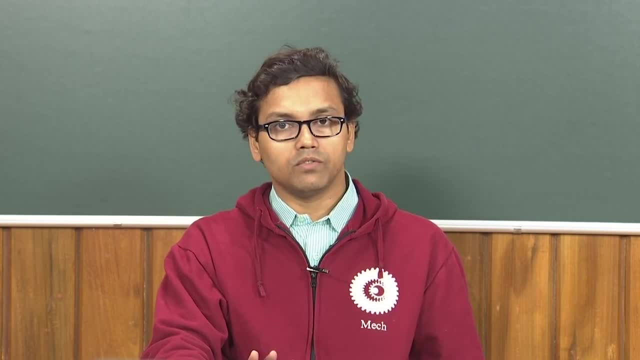 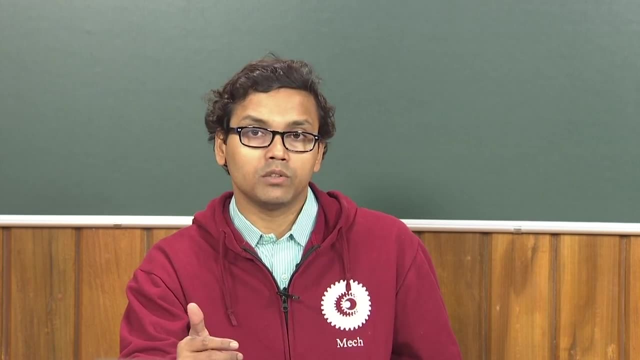 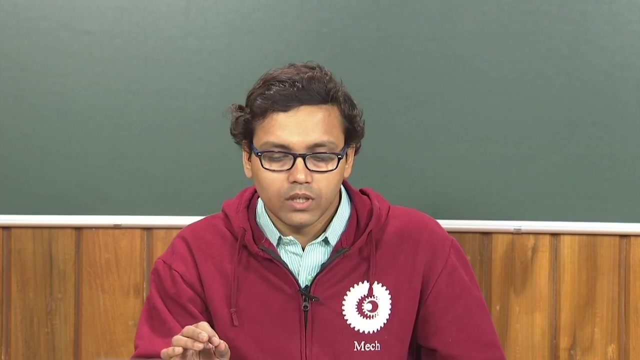 called cladding and therefore the energy that is produced inside the fuel. if you are particularly talking about a solid fuel, the energy produced inside the solid fuel. that will get conducted through the solid, from its center line to the wall and from the wall of the fuel. the cladding is there So that heat has to be conducted through the cladding. 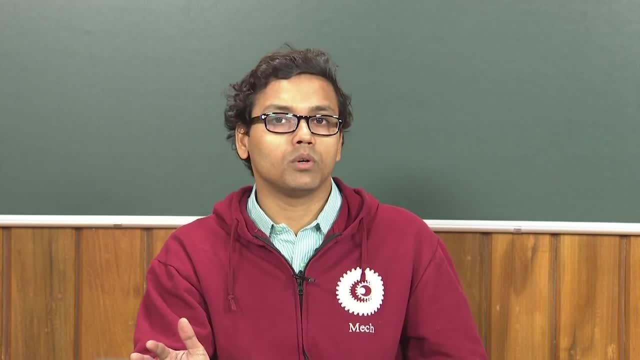 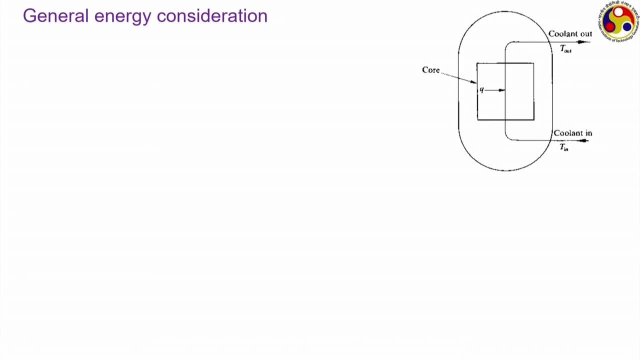 material as well, and then only it will be able to come in contact with the coolant. Now this is brief schematic representation. if q is the amount of energy that has been produced by the core and if coolant is coming with some temperature and going out at some 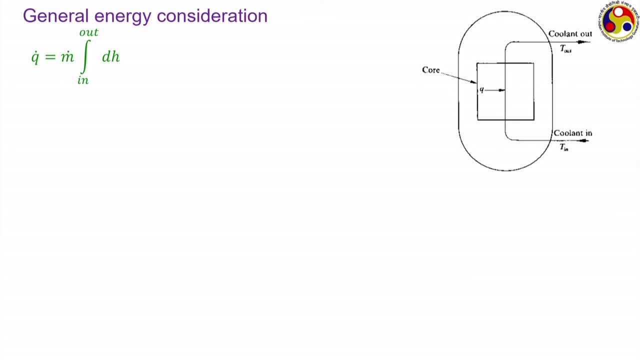 elevated temperature. then we can write a simple energy Energy balance: is q dot equal to m dot into integral of d h, where q dot is the power production rate and m dot is the mass flow rate of the coolant, and hence it is m dot. 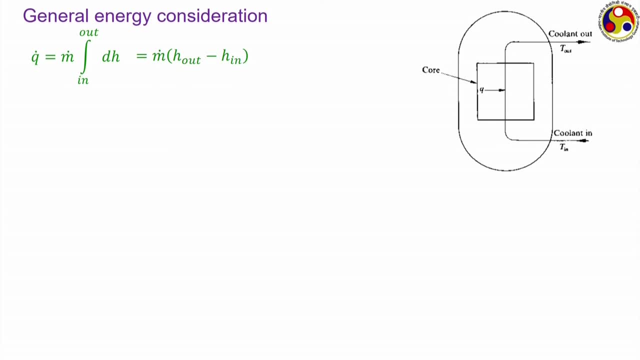 into h, out minus h, in assuming that m dot remains constant. This is, of course under steady state. this energy balance has been written. If the coolant retains the single phase status throughout this passage, then we can always write this thing because we know, as per the definition of specific energy balance. So the energy balance is q dot equal. 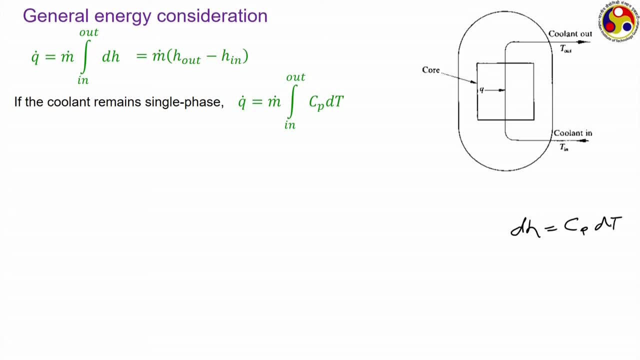 to m dot into integral of d h, where q dot is the power production rate and m dot is the specific heat. d h equal to C p, d t or C p is equal to dou h, dou t at constant pressure. and that is why we can, for single phase situation, we can write this way: If C p remains constant, 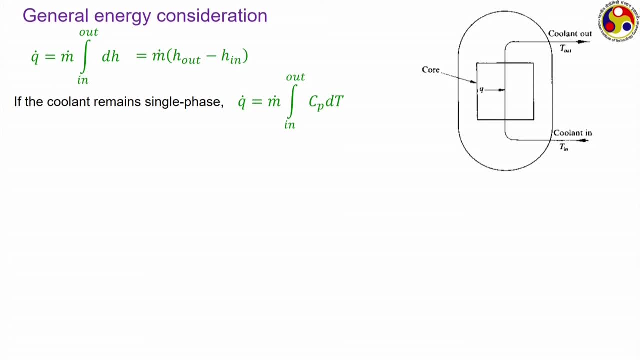 this is a very straightforward integration but generally C? p is a strong function of time. particularly at higher temperature that can show a quadratic kind of relationship. Now let us take a look at this particular chart. We have earlier mentioned that the energy balance is the mass flow rate of the coolant which has been converted to the vapor. 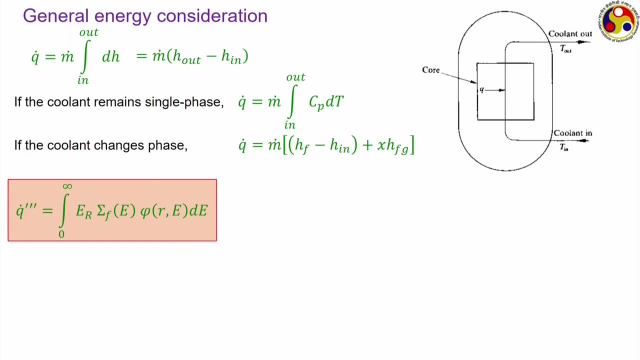 phase. Now this expression we have found earlier: energy released by because of fission per unit volume can be given expression like this: where E, r is the amount of energy released because of fission, sigma f is the macroscopic cross section, phi is the flux distribution. 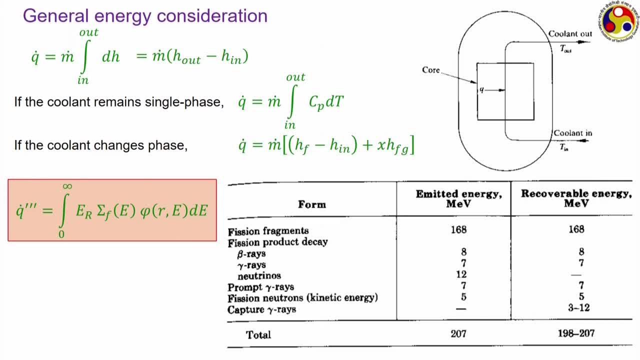 by the neutron. Now let us take a look at this particular chart. We have earlier mentioned that the mass flow rate of the coolant which has been converted to the vapor phase, So we can see that the because of fission reaction there is about 200 MeV, slightly greater than. 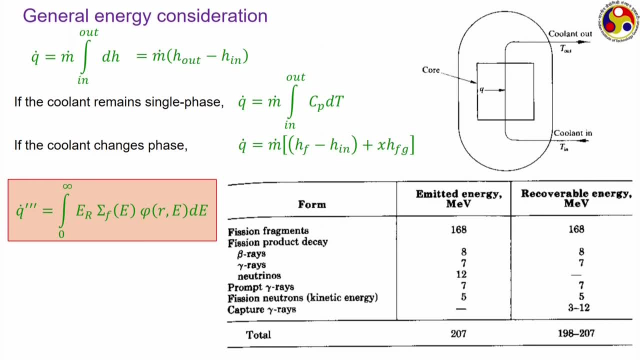 200 MeV. actually, amount of energy is released, which corresponds to the mass defect, But how that energy is being transmitted. Of course the fission fragments take care of the majority part of that, which is about 160 MeV, but there can be several other components like fission. 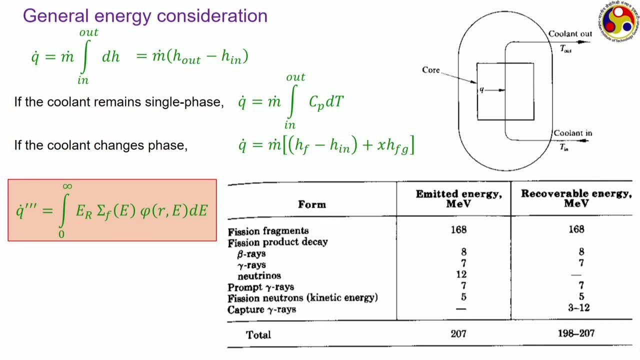 energy carried by the beta and gamma rays or by the neutrinos, The fission, and also, So there can be a significant amount of energy carried by the gamma rays which are released during this reaction. but out of this, all this possible contribution, actually this 168. 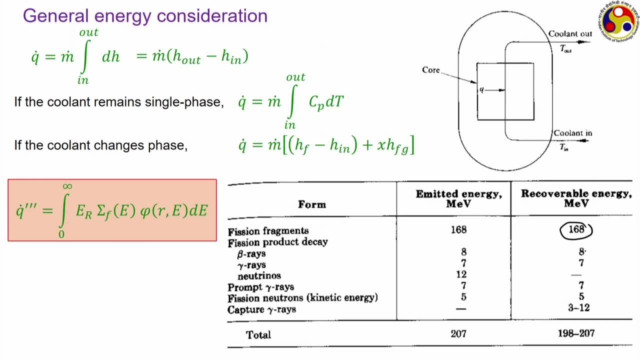 MeV from the fission fragments and this first 8 MeV from the beta rays combined together are usable or available as thermal energy. Rest are available, either energy through radiation or by some other means, something like delayed neutron decay, etcetera, And hence, while we had a total figure of 207 to deal with for this year, practical case: 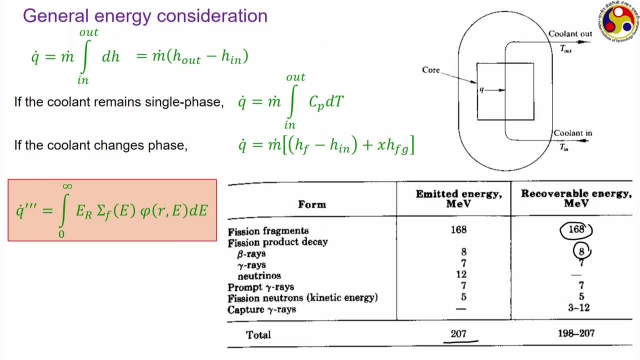 we are going to get only about 80 percent of that, and hence this year must be substituted with an effective value of that which, come generally, is about 80 percent of this theoretical level, And hence we can perform this integration as an approximate summation. 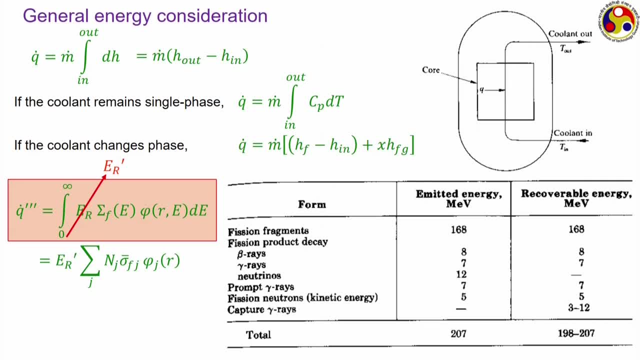 Where we are considering, say g, m, multiple groups of the neutron flask. So E r prime, being a constant, is outside the integration, and here g refers to, here j is the each of the small neutron groups that we consider like. if we remember from the previous module that in a reactor we can have several groups of neutron neutrons which 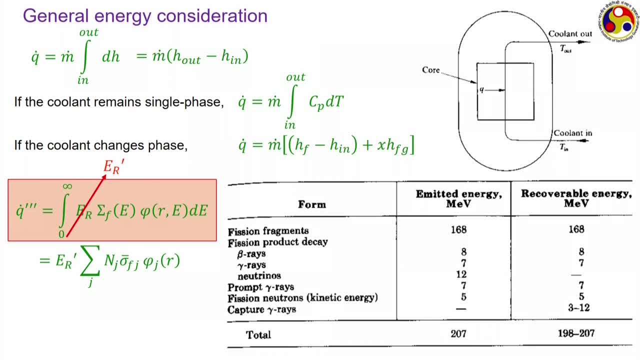 σk is probability of water refektion. So here which I am looking at, that multiple groups of the neutrons flask, Where we are considering, say, g, m, multiple groups of the neutron flux, neutrons, And therefore we often adopt a multi group approach, that is, we divide those. 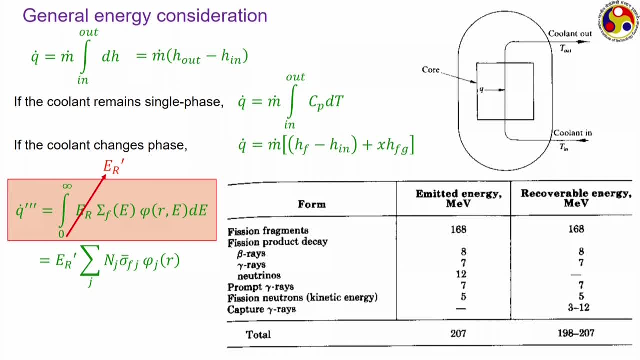 neutrons into several groups and some there, and perform the calculation for each of them and then some that over the entire range of energy available, and the same has been shown here. Here G refers to any particular such group. N, j is the total number of nuclei present. 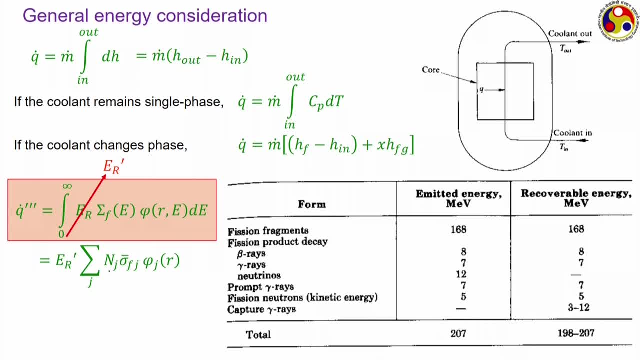 there and sigma f j is the average fission, microscopic fission cross section under that group and phi, of course, is the neutron distribution of that energy level. We already spend lots of time in the previous module discussing the distribution of this phi, and let us take 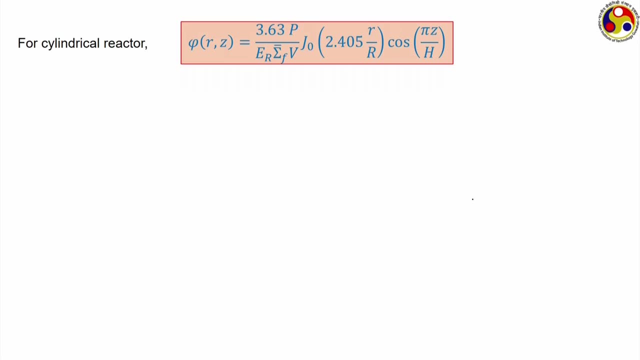 one result from there. This is the one result that was shown there for a cylindrical reactor or a cylindrical fuel element. Here this j naught is the. here this particular j naught is the Bessel function. ok, Er is the energy released during fission. that 200 MeV, the order of, and this one the sigma. 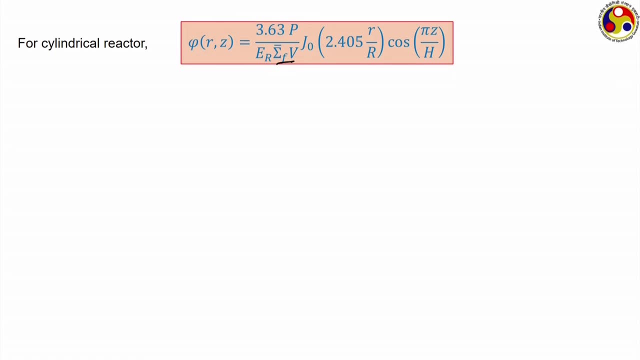 f bar is the averaged fission cross section of the reactor, P is the power production or power rating of the reactor and this V is the volume of the entire reactor. So capital R refers to the radius of the cylinder and capital H refers to the height of the cylinder. 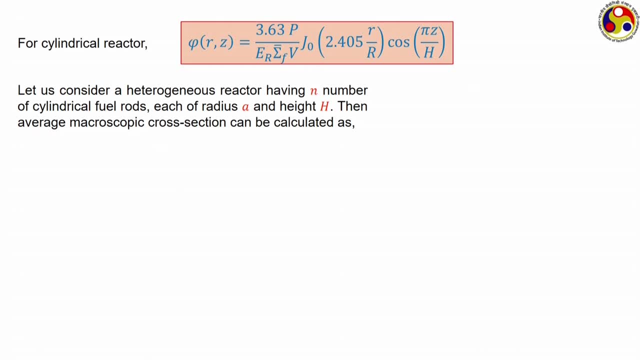 Now let us consider a heterogeneous reactor which has small N, j And number of cylindrical fuel rods, So each rod can be viewed like a cylindrical reactor, kind, kind of kind. and each of these rods are having a radius of small a and height of h. 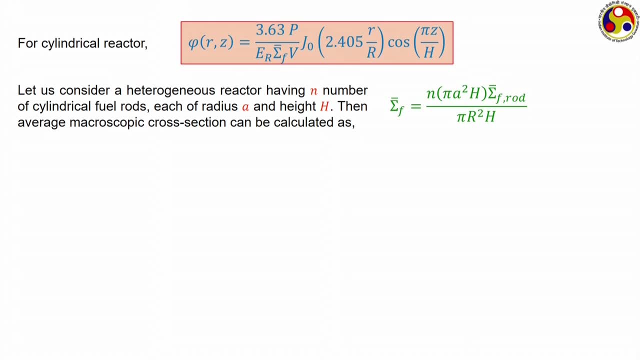 Then the average macroscopic cross section can be calculated like this: where pi square h is the volume of each fuel rod, multiplied by N gives you a total volume of all the fuel rods, and pi R square h is the volume of the reactor itself, Soby we can simplify this as a form like this: Now, if we put this expression for sigma, 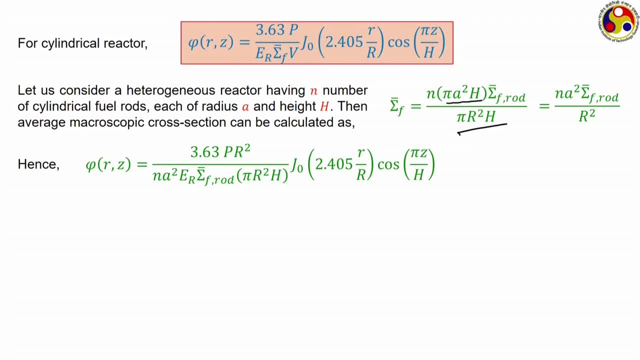 F in the above expression. then we get like this, which finally simplifies to a form like this, So finally put in this expression for five in the previousah slides expression, we get the volumetric rate of energy generation of a form like this Here. just note that here and here prime both a fears, where this here. refers to these gave us So, as would be fit here, x, So suchl, the formation that e and r h looks like the expression: error of n d f differentiation. error of n? d f differentiation. finally, the equation solved, this expression, which will give the Stress equation into we. 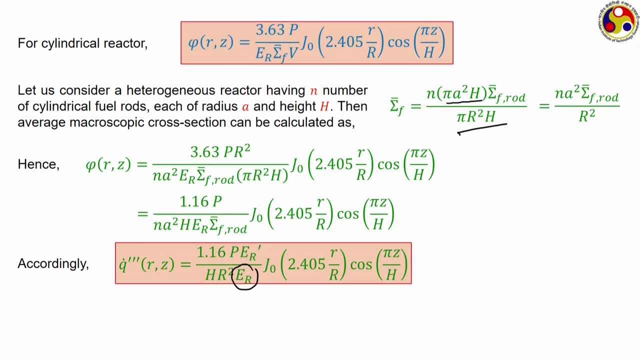 then we will be able to refer to that v sincerely. just remember to first let me such that amount of energy released during a single fission reaction. this is a theoretical value And E? r prime is the effective value of that E? r which can be recovered in the form of. 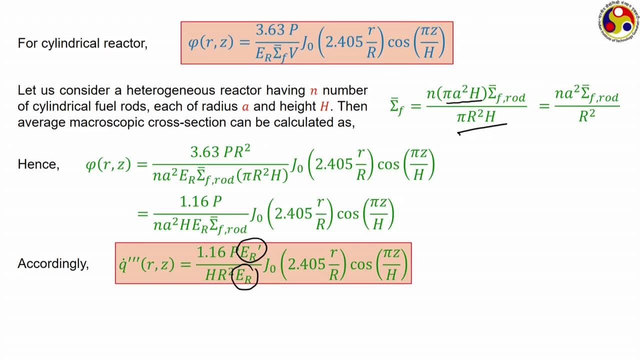 thermal energy. But still we are using this E r in the denominator because while calculating the power rating for a reactor, generally the E r is used As E r prime. E r is more or less constant, but E r prime that may vary from one situation to another. So like say this: 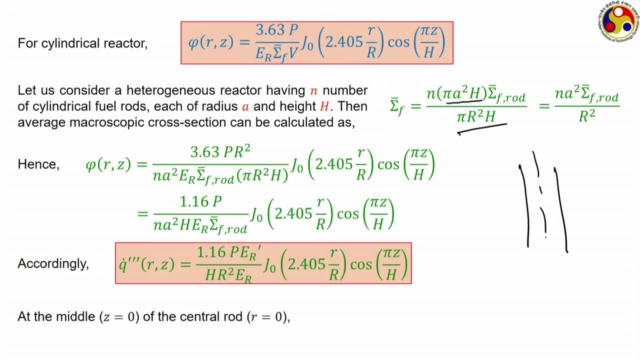 is our reactor, the cylindrical reactor. this is the center line. we are taking this as a coordinate system. So center line refers r equal to 0 in the vertical direction. also, let us take the middle of the core cylinder as the coordinate system. So here z starts. 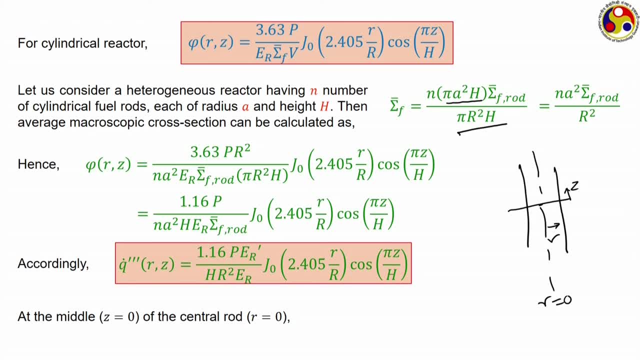 from here, And hence we are taking this as a coordinate system. So here z starts from here, and hence we are taking this as a coordinate system. So here z starts from here, and hence we are put r equal to 0 and z equal to 0 in this expression, that is, if you are talking about. 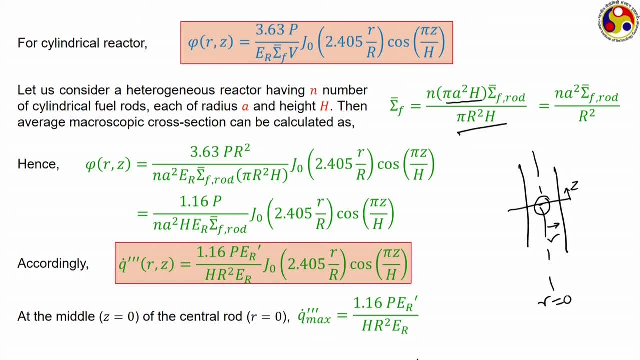 this particular location. then it reduces to a form like this: Actually, cos 0 is equal to 1 and z naught 0 is also equal to 1.. It asymptotically approaches 1.. So we get this as the expression of the maximum volumetric rate of heat generation and putting that the 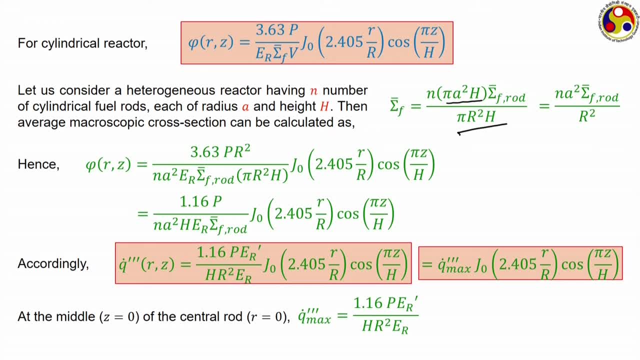 final expression gets simplified to a form like this. This way, by knowing the nature of the medium and nature of the heterogeneous medium, and also the using the standard solutions, we can always calculate the total amount of energy that is available to be transferred to the coolant. 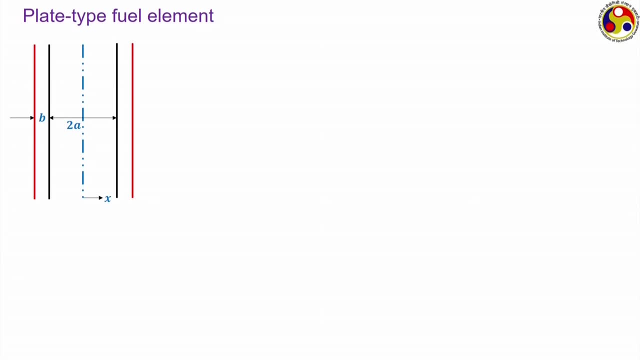 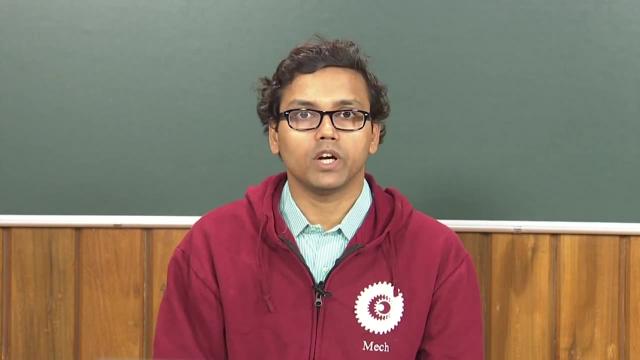 So let us take or consider a couple of simple situations. Our first case is that of a plate type fuel element. as I have mentioned, commonly reactors have two kinds of fuel pellets. one is of a plate kind, other is cylindrical or fuel rod. 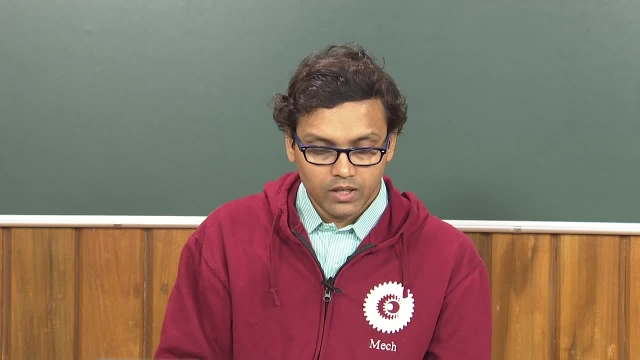 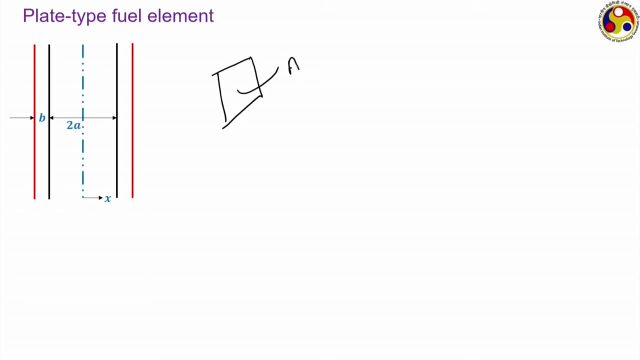 So here we have a plate type fuel element of thickness 2 a it is, which is not possible to show in the diagram. it is cross section area. we are taking as capital A cross section which is perpendicular to this slide and on both sides this element is covered by a cladding. 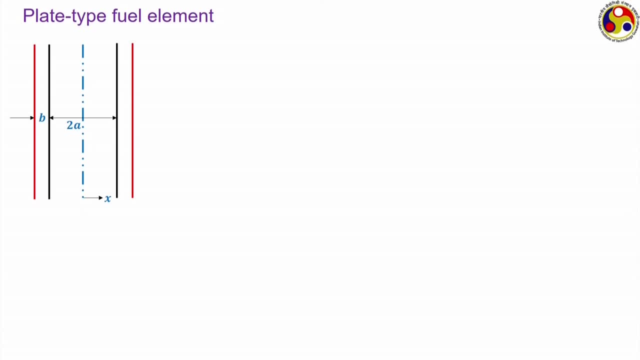 of thickness b. Now generally, in general reactors, we will find that this dimension 2 a is extremely small compared to the dimension in the other two directions, and hence it can be considered to be, or it can be viewed as a one dimensional problem. 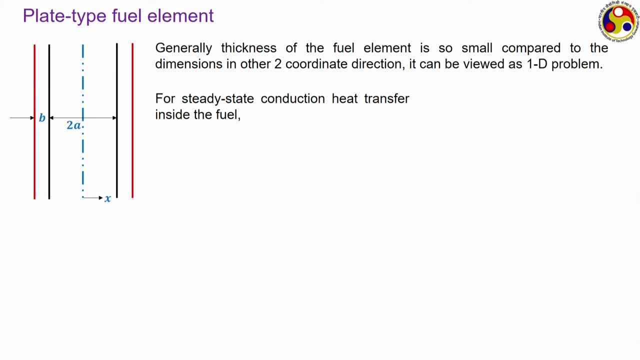 So, under steady state, the heat transfer in the fuel can be written, can be written following the Cartesian coordinate system. it can be written like this, Just I repeat here: conduction is the only mechanism that is happening inside the fuel, this being a solid. 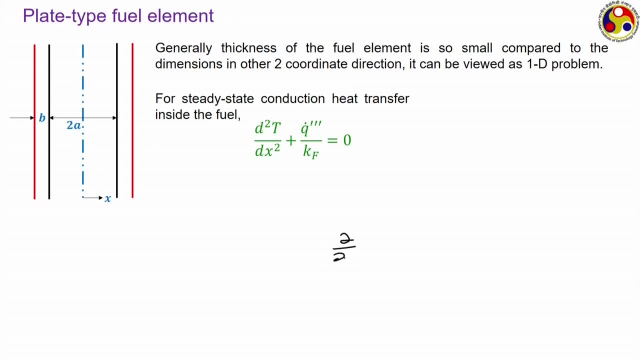 And now the generalized heat conduction equation in 3D Cartesian coordinate can be written as: 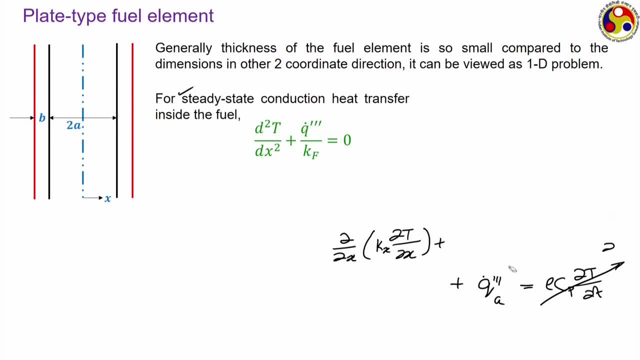 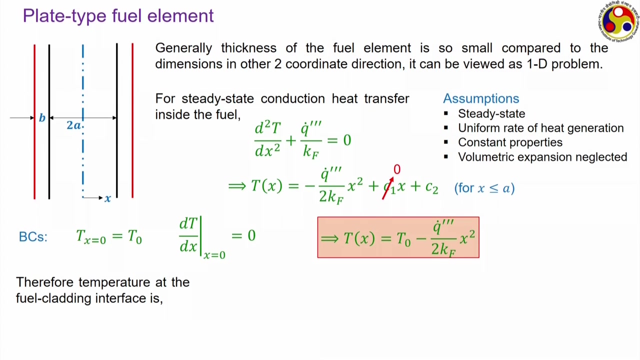 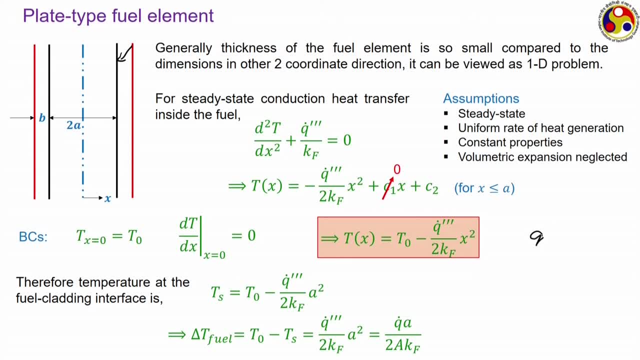 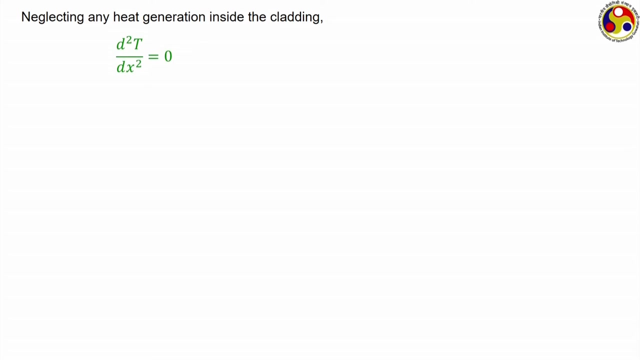 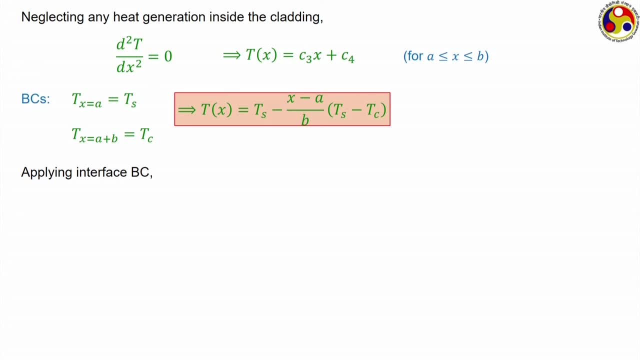 heat transfer. both the temperature and the temperature gradient or the rate of heat transfer should be identical at the interface of the fuel and the cladding. That means at x equal to a T or temperature should have a continuity and there is same condition we are using here. 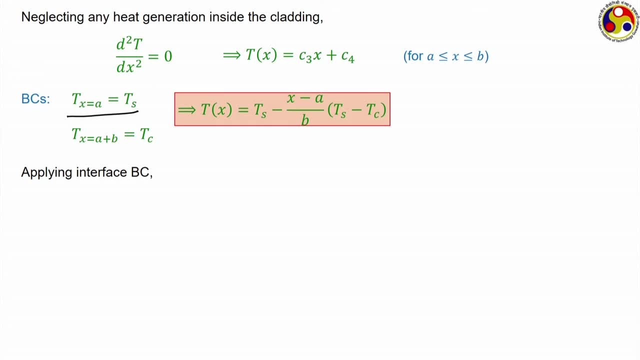 at x equal to a, T is equal to T, s for both cladding and fuel, And here we can use the second condition, that is, the rate of heat transfer. conduction is only mode of heat transfer here, because both fuel and cladding are solids. So minus k. 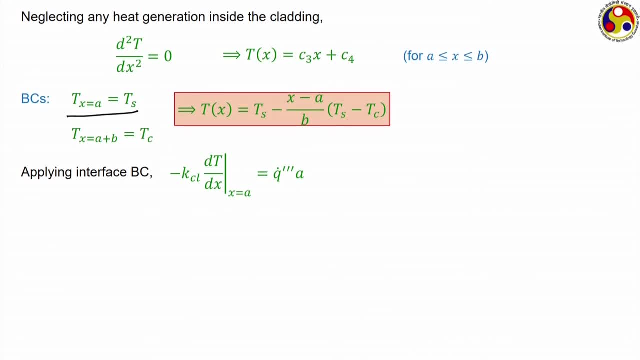 dT. dx at x equal to a should be equal to the total amount of heat flask that is getting transmitted through that phase. Here we have used the Fourier's law of heat conduction and the heat flux. just that is coming out through one of the phases. Let me write it. 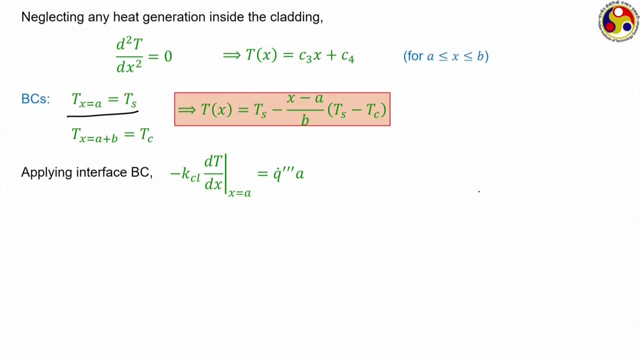 in a better way. The heat flux coming out of one of the phases should be equal to the energy produced in that half of the reactor that is, as we have seen into previous, slide to a divided by the cross-section area. that is why we are having this term here Now, using this interface boundary condition. we 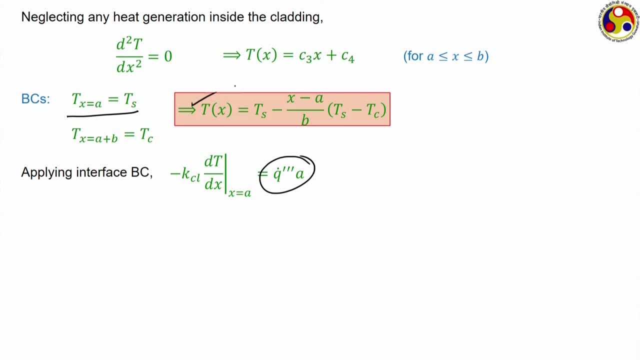 can calculate, we can derive, we can get the derivative of this and put the condition x equal to a And consequently we get the temperature change across. the cladding, that is T s minus T c, should be of a form like this: q dot b by a into k, c, l. So again drawing the thermal. 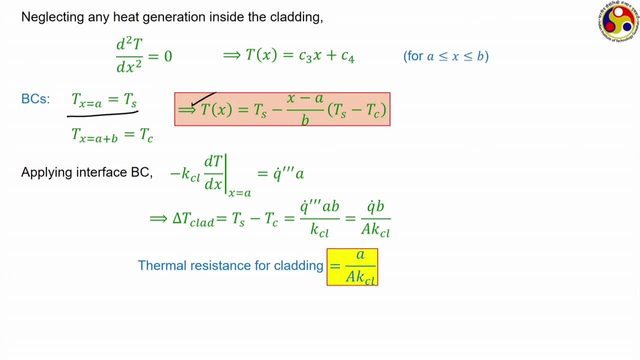 energy. we can define a thermal resistance for the cladding as small e, divided by a into k, c, l. Finally, the energy that has reached the cladding must go to the coolant stream, which is flowing on the surface of the cladding, along the surface of the cladding and there. 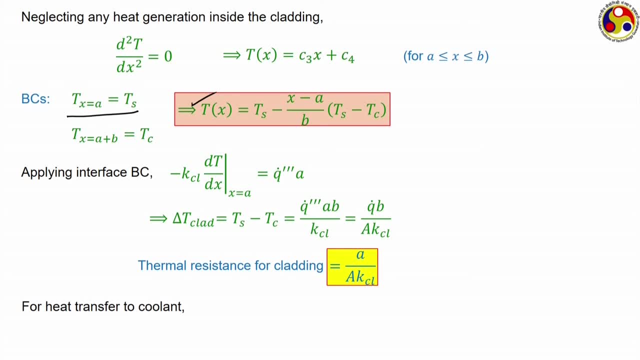 the mode of heat transfer is convection. So now we have a surface here and there the temperature. we can write a general energy balance between the cladding at the cladding surface. that is the amount of conduction. heat received by the cladding should be equal to the amount. 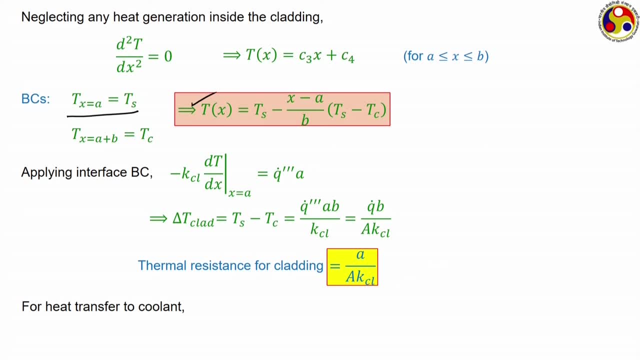 of heat transfer to the coolant via convection under steady state, And hence the total rate of energy generation by half of the reactor should be equal to h A into T c minus T bulk. here small h is the corresponding heat transfer coefficient And accordingly we candefine a flim heat transferflim temperature difference delta. 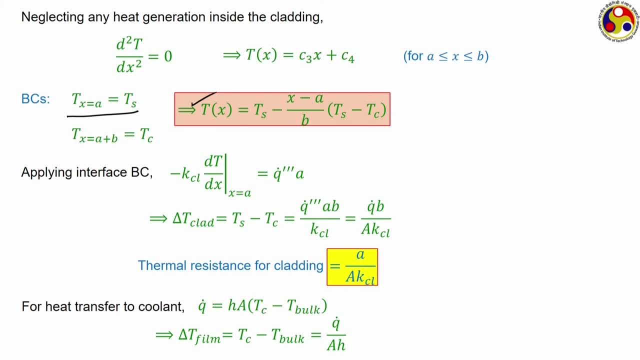 T flim as the temperature difference between T, c and T bulk, and that is found to be q dot by a h. So we can define a thermal resistance for the flim as 1 upon h, which is actually the very standard form of thermal resistance for convection in Cartesian coordinate. 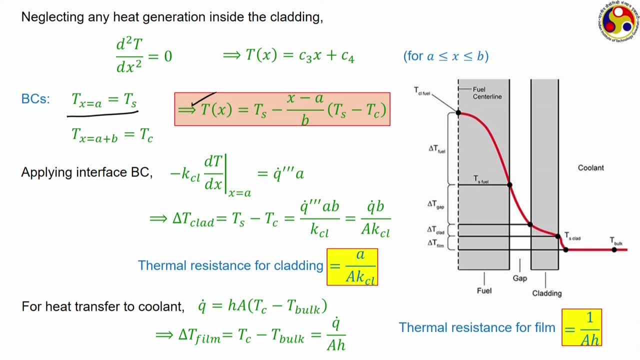 This is a typicaltemperature profile that we may have actually in reactors. you may find that the fuel and cladding cladding are separated by small air gap or gap over by some kind of ah inner, some kind of inert gas. So inside the fuel we are getting this kind. 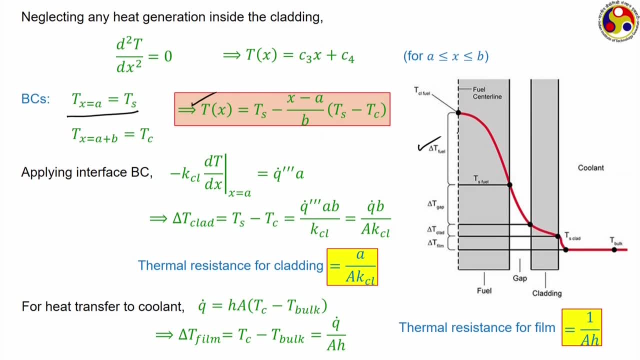 of temperature profile and this is the temperature change across the fuel. This is the temperature change across the cladding and if the gap is there, we are going to have a temperature change across this as well. And finally, this is the temperature change across the. 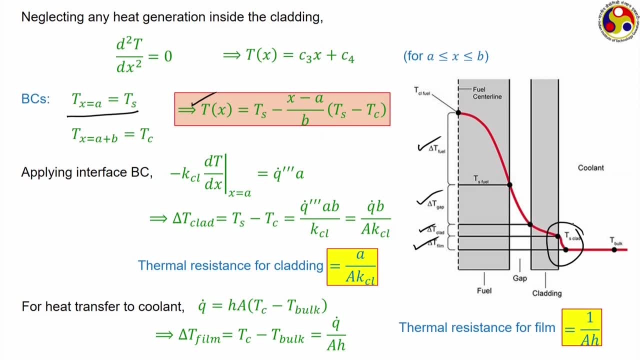 liquid flame, This portion, the flame of liquid which may get generated on the outer surface of this build, outer surface of of this cladding. So we shall be doing that in the next lecture again. but as we have already calculated the threeheat transfer resistances, So the we can also combine them to get a combined 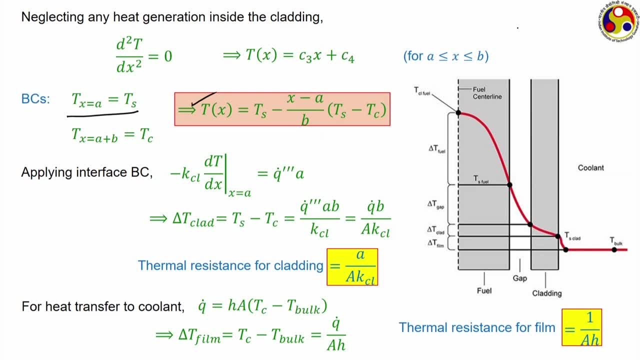 expression of total temperature change across the fuel. So the temperature difference- that is the reason for having such a heat transfer, which is the difference between temperature at this particular point and the bulk temperature, So T naught minus T bulk, divided by heat transfer should be equal to the summation. 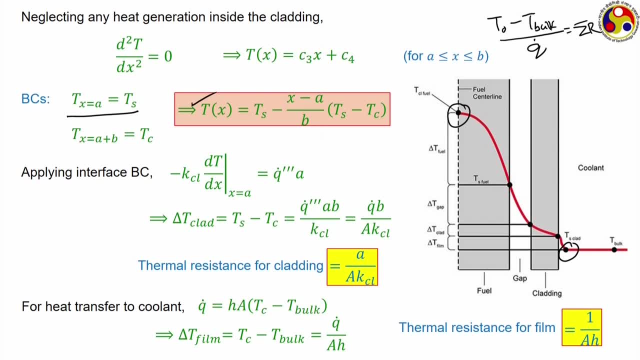 of all these resistances, We have already calculate the resistance corresponding with the fuel, the cladding and the coolant- or heat coolant film, I should say- And if there is a gap between the heat transfer and the heat transfer. So we have already calculated. 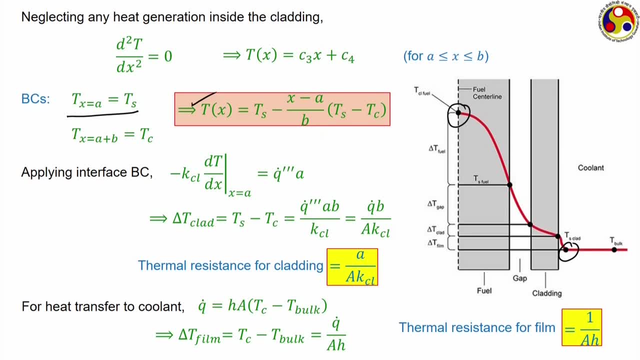 the resistance corresponding with the fuel, the cladding and the coolant, or heat coolant film, I should say. And if there is a gap is involved, then we can also calculate the resistance for that gap and add to this We can perform analysis of a cylindrical fuel. 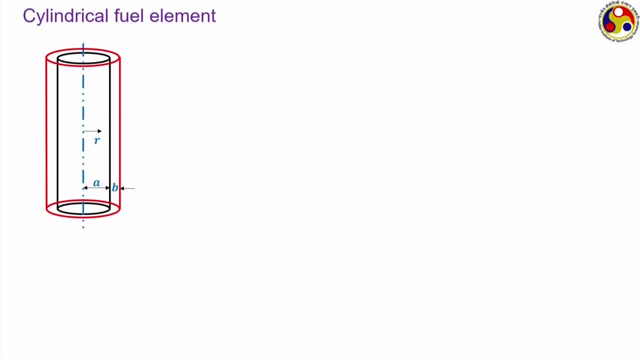 element. the same way. Here we have a cylindrical fuel pin of radius small a and there is a cladding covering of the around the cylinder which is having a thickness of small b. Here we can perform the similar analysis, but following the cylindrical coordinate system. 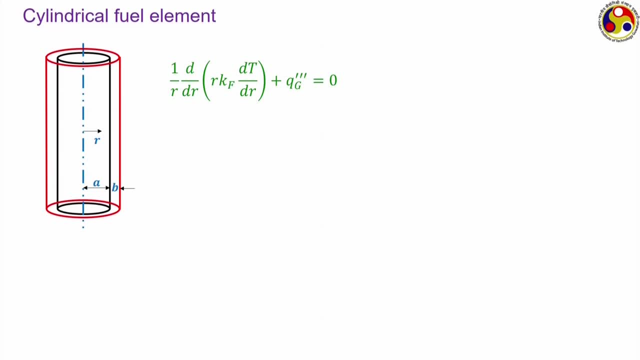 So this is the one dimensional steady state heat conduction equation in cylindrical coordinate system, And by solving this we are here and then integrating it once more, we are getting in this particular temperature profile inside the cylinder, that is, for r less equal to a. 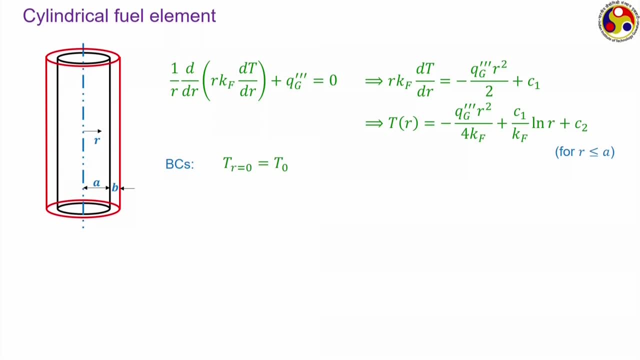 Now we need to use the boundary conditions, Similar boundary conditions. at r equal to 0, the temperature is T naught, which is centerline temperature, and again, centerline being a plane of symmetry, the temperature gradient will be 0 as well. So putting the second condition, 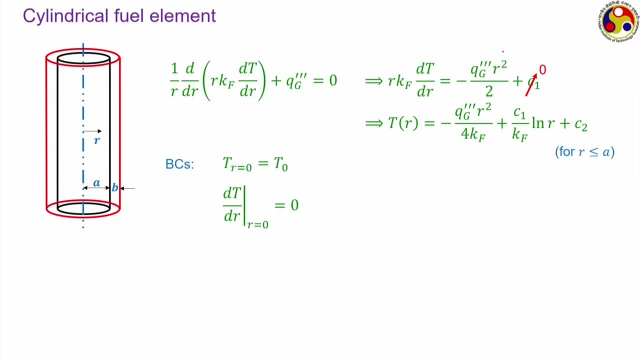 we can straight away say that c 1 equal to 0, Like if we put r equal to 0 here and dt d r equal to 0 here, c 1 has to be a 0 And then puttingthis other second boundary condition. 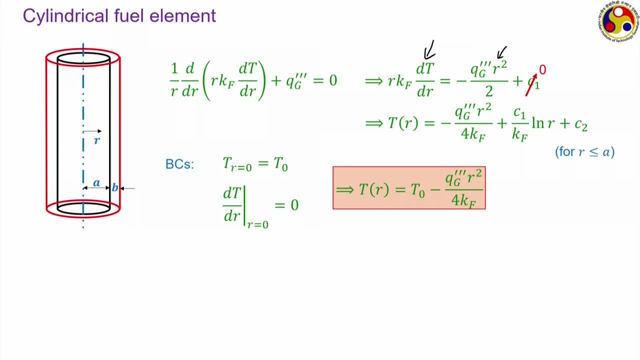 in the remaining expression we get c 2 equal to T naught and accordingly this is the responding temperature profile. Therefore, temperature at the fuel cladding interface, where r equal to a, if you need to put, we are getting the corresponding expression and hence the temperature. 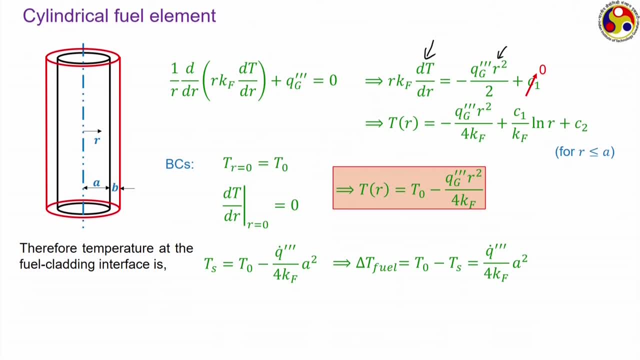 difference across the fuel is q dot triple prime by 4 k f, a square Rate of energy generation inside the rod. So we can write: the temperature difference can be given by like this: Why pi a square h is the volume of this rod and q dot triple. 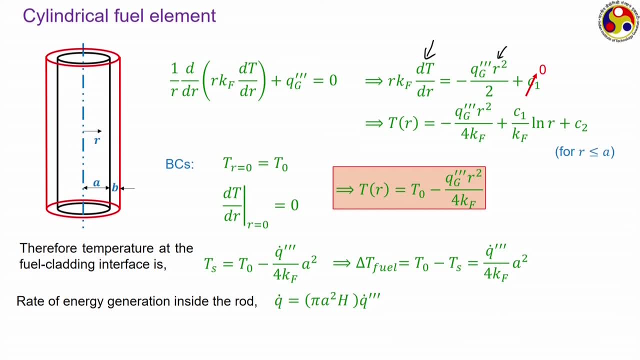 prime is the rate of energy generation volume. So if we use this definition in the previous expression, the temperature difference can be written like this: And now we can again draw the electrical energy to get the thermal resistance for the fuel which actually will be this delta T divided by q, dot So is equal to 1, So we can. 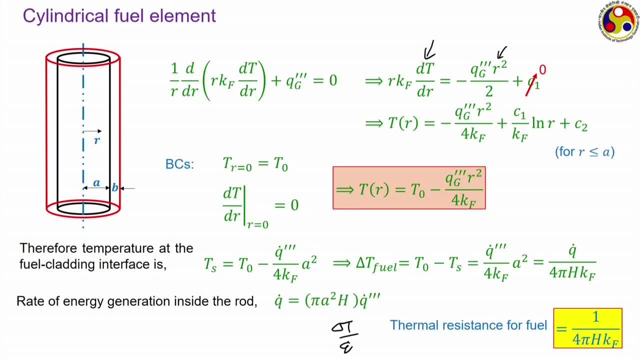 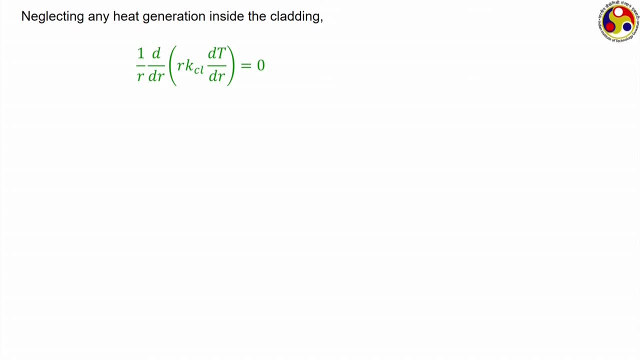 write the thermal resistance as 1 by 4 pi h into k f, where h is the height of this cylinder that we are talking about, Again neglecting heat generation inside the cladding. we are having this simplified expression, And then we can integrate this this way Now. 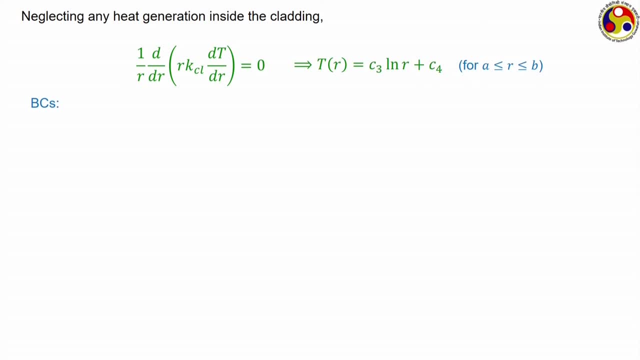 the boundary condition can be to specify temperature. on both side of the cladding There is T at r equal to a is equal to Ts, And the second condition at the other edge of the cladding, that is r equal to a plus b, T is equal to T c. So if we combine them we get this phi. 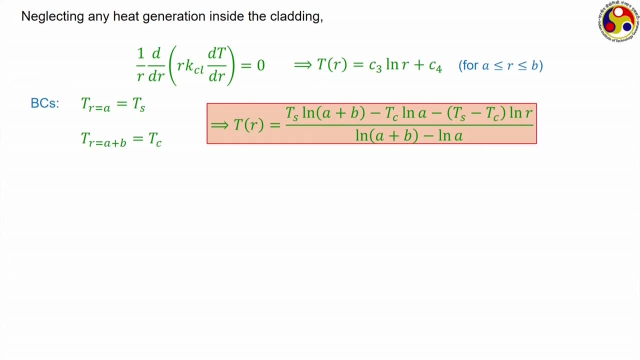 particular expression. I would request you to derive this on your own. This looks complicated, but actually can be quite simple. And now again we apply the interface boundary condition, that is, the total amount of energy that has been produced by the fuel that must pass through. 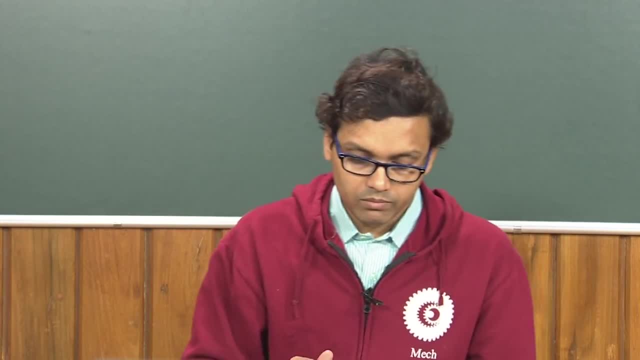 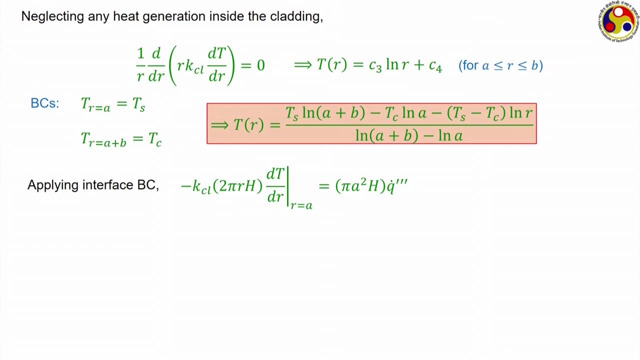 the cladding itself. So k dot t, dou, h, dou r at r, equal to a, into the area. corresponding area should be equal to the amount of energy produced inside the cladding. Here 2 pi r h refers to the area of the cylindrical element at any radius r and h is the height And accordingly 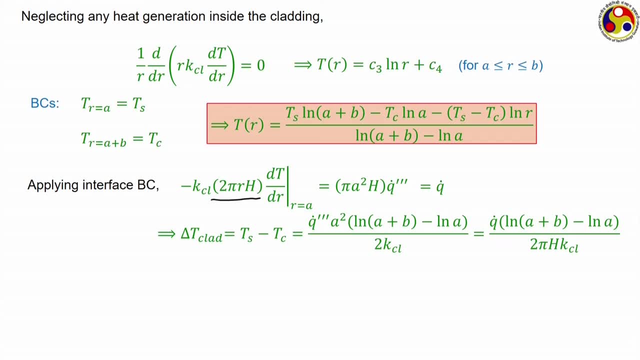 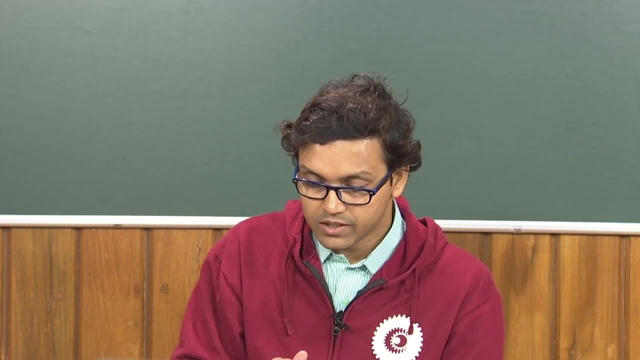 we get the temperature difference across the cladding is equal to k dot into log a plus b, minus log a by 2 pi h, k, c, l, And hence we can define a thermal resistance for the cladding as this log of a plus b, minus log a by 2 pi h into k, c, l. And finally, again, we can define 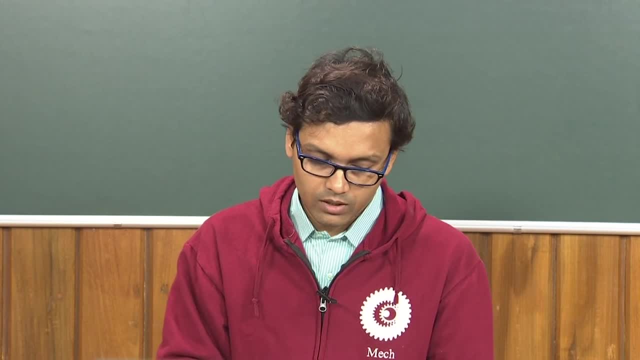 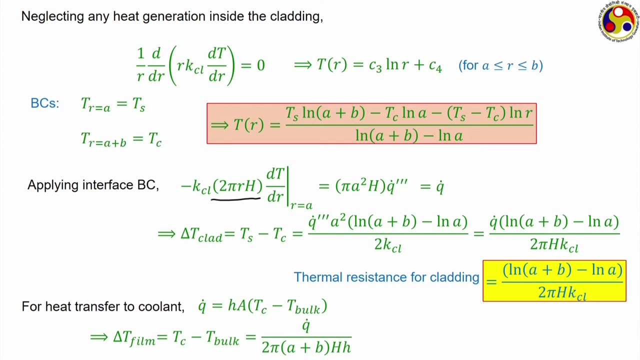 a thermal resistance corresponding to a convective heat transfer to the coolant by equating the energy transfer, So heat transfer from the cladding to the energy received by the coolant. small h again is the heat transfer coefficient And hence we can define a film temperature difference. 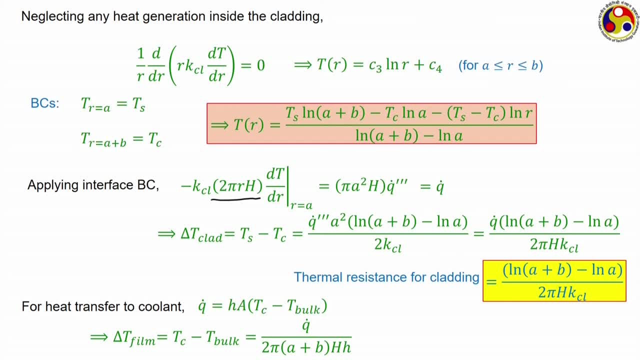 as q dot by 2 pi a plus b into h, into small h. So the corresponding thermal resistance for the film is this. Hence, like in case of a planar element, for cylindrical element also, we have identified the three thermal resistances, Of course by assuming the properties to be. 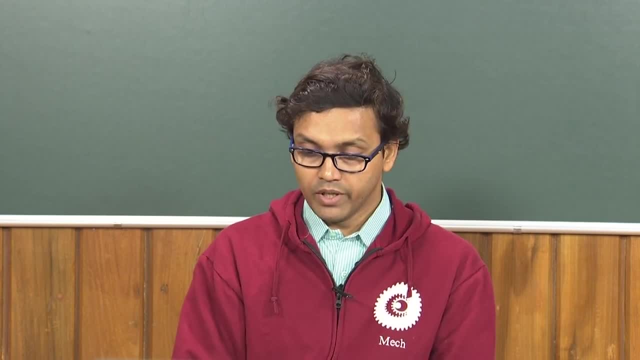 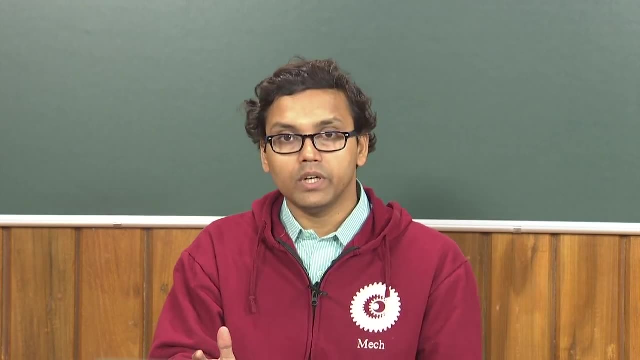 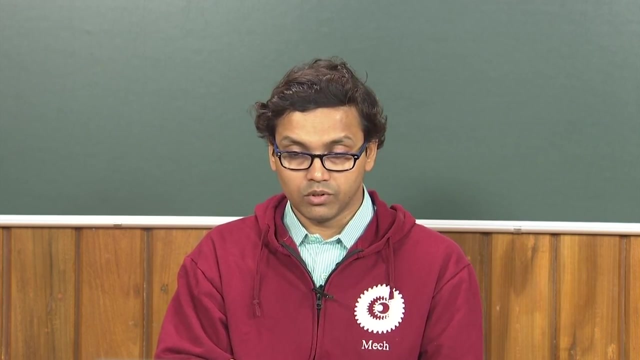 constant property, like the k f and k c l. If we assume them to be constant, then we know how to calculate the three thermal resistances And accordingly we can calculate either the bulk temperature if we have knowledge about the central in temperature, or the central temperature if we know, if we somehow identify. 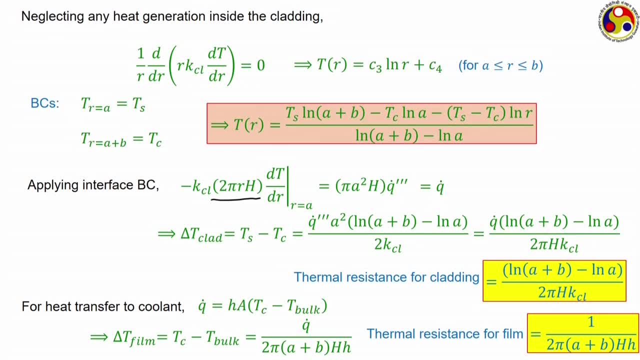 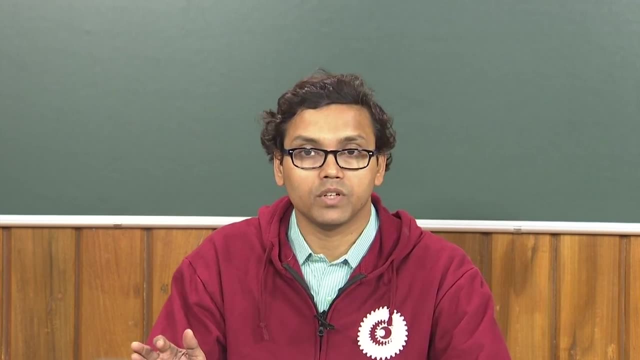 all these three. So if we can calculate the or measure the bulk fluid temperature, which is not very difficult, One problem, of course, will be this small h, the convective heat transfer coefficient, which depends on the properties and also the velocity level of the coolant. 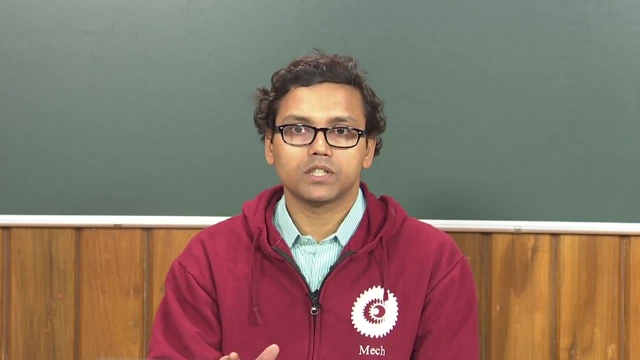 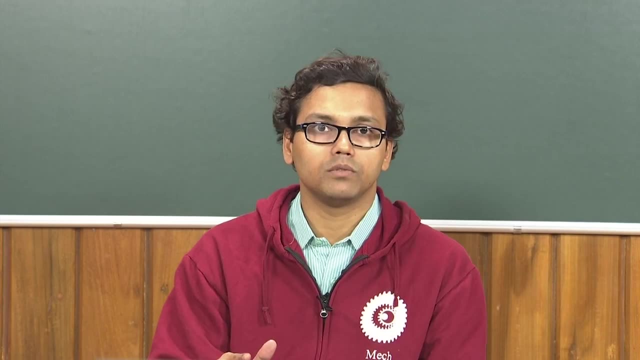 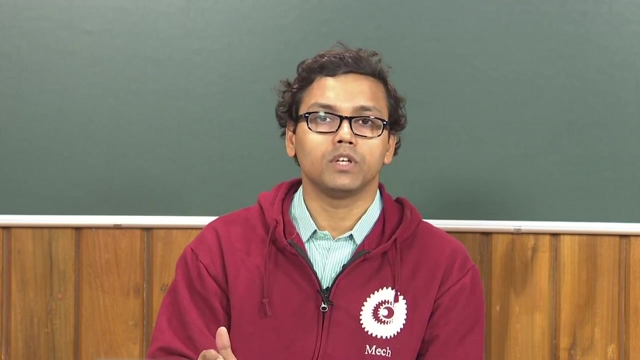 stream itself. ah, But the two geometries that we have discussed here, both are quite simple, like one important assumption was the uniform heat generation that we are having inside the react fluid element, which practically is not true. Like in the previous module, already we have seen that neutron flux can have quite complicated distribution over the reactor. 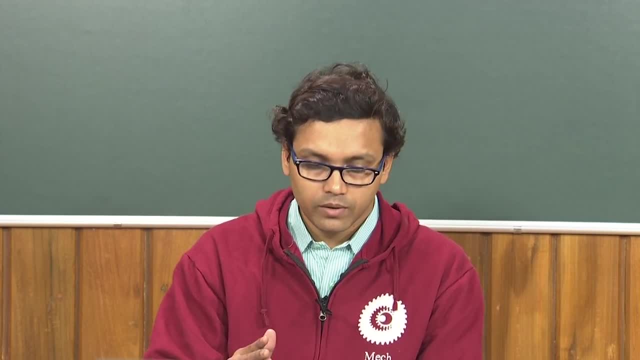 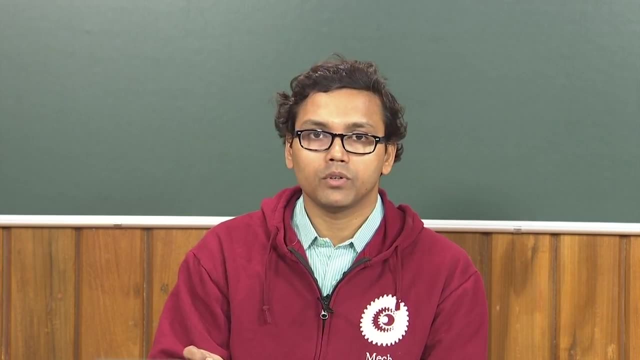 and if the neutron flux is varying then the ah- heat generation- has to vary in proportion. So in the next lecture we shall be taking it from this point onwards where this thermal resistance values will be utilized, but we shall be considering the neutron flux to be 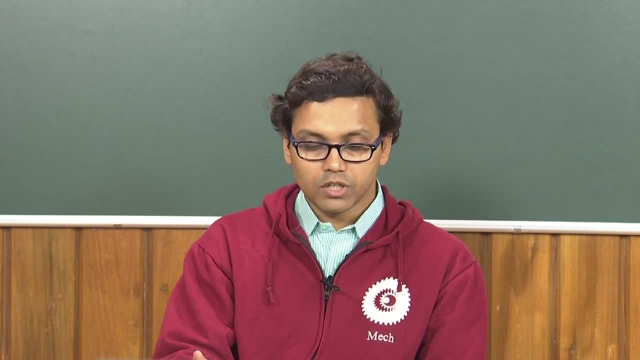 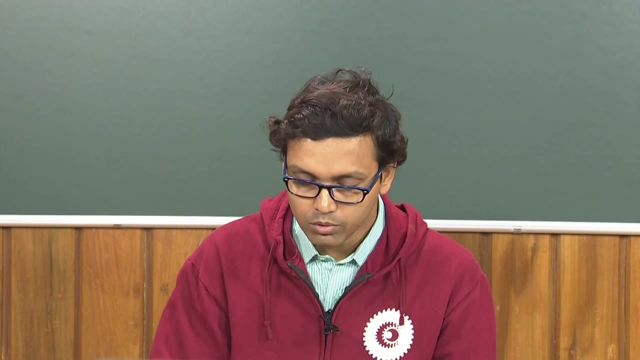 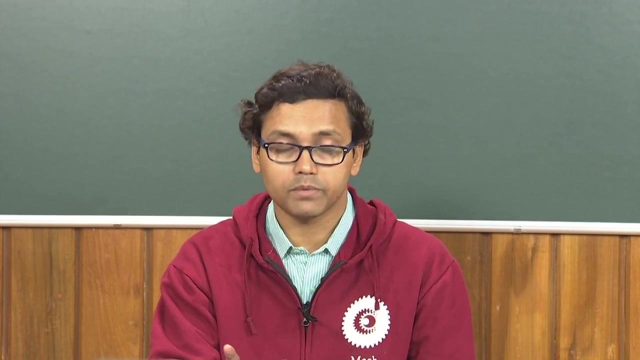 varying, and so, ah, thereby we shall be able to do a more complicated and involved heat transfer analysis. So, ah, I am leaving this up to today. please go through the analysis and go to through all these derivations. I would request you to derive on it, all these steps on your. 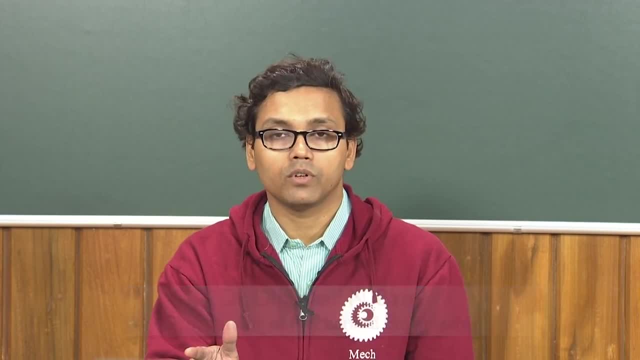 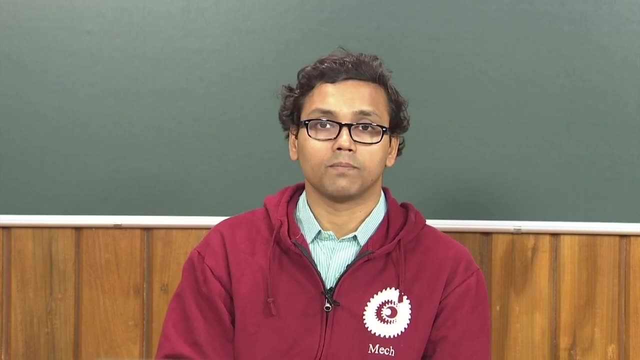 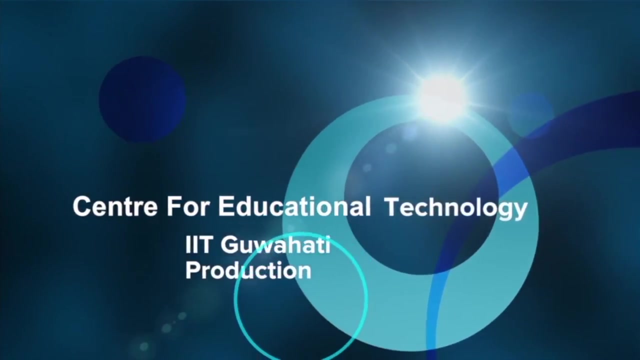 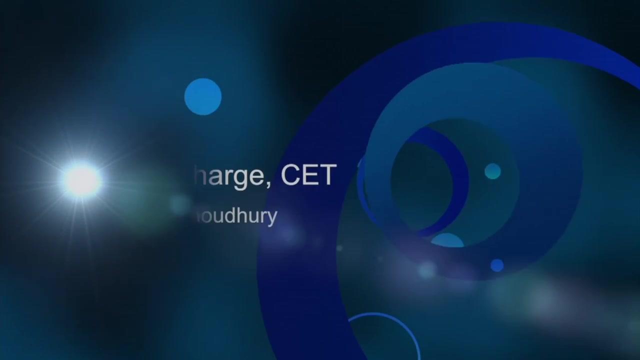 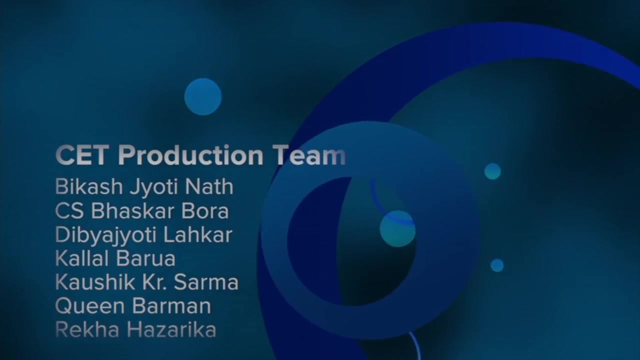 own And so that when you come for the next lecture, you know all the intermediate stress and you know how we are derivingevery term this. So thanks and bye for that.